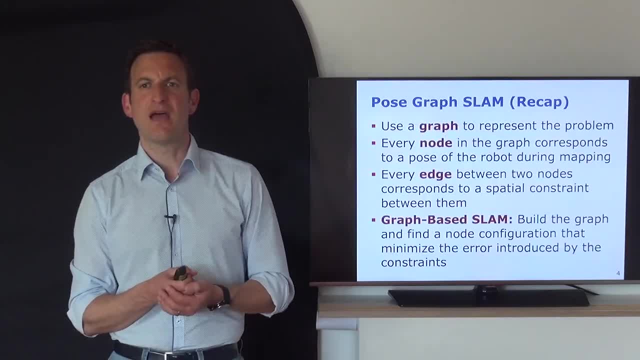 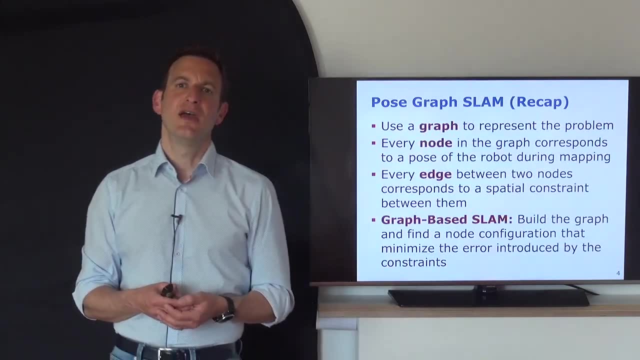 And so the key idea of the postgraph was to have a graph where every node in the graph consists of a post that the robot has been at a certain point in time during the mapping process, and every edge in this graph represents spatial constraints between those nodes. 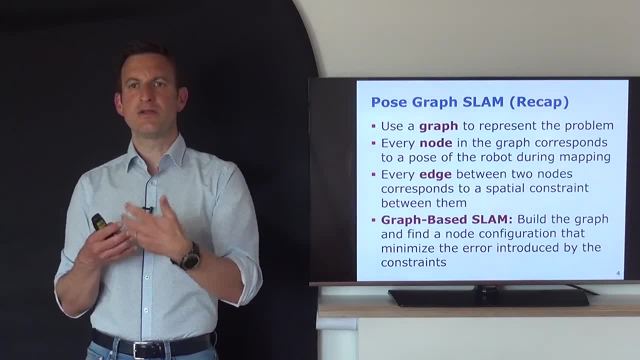 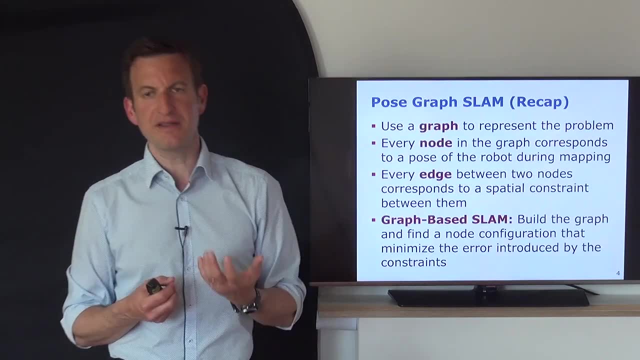 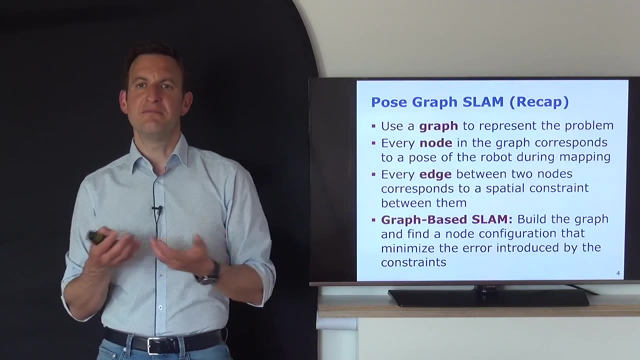 So it's typically a relative transformation- how one node can be transformed into a second, Or relative constraints between them, And the overall idea of this postgraph-based SLAM is to find a configuration of those nodes in the graph that minimizes the error introduced by the constraints, because those spatial constraints may act against each other. 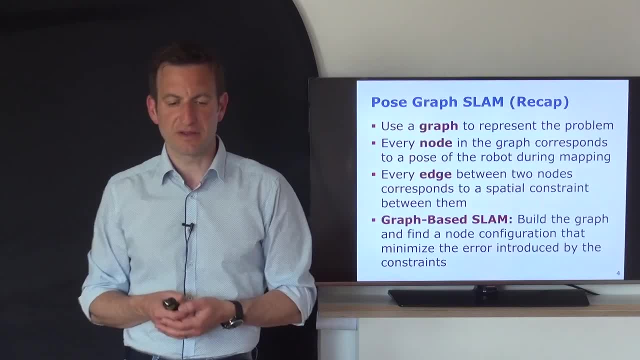 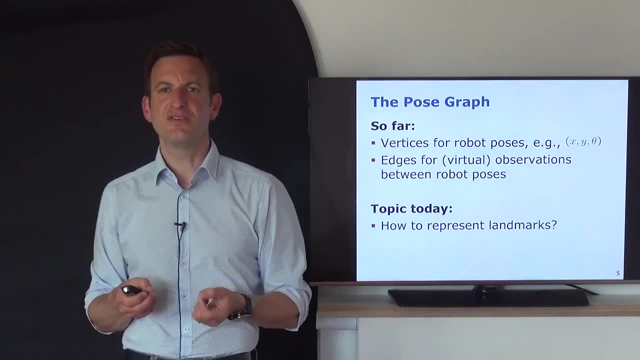 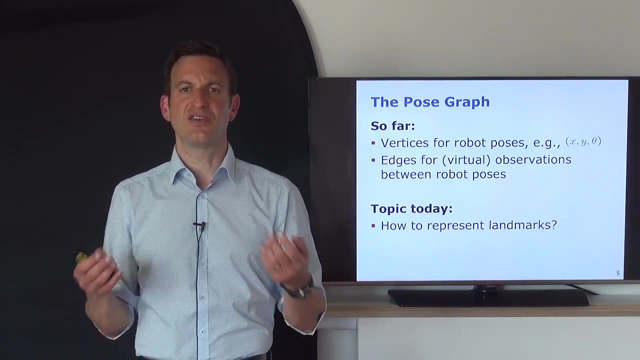 This results from sensor noise and also from maybe imperfect data associations, And so this was done with the so-called postgraph. So in this postgraph the vertices or nodes were always robot poses, So X, Y and orientation theta for the 2D case, or X, Y, Z and three rotational angle Yaw-Pitch-Roll, for example in the three-dimensional case. 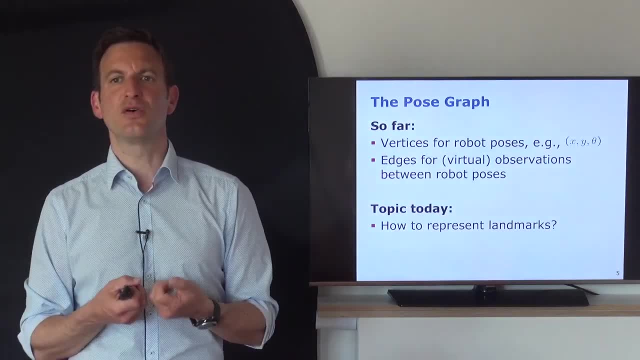 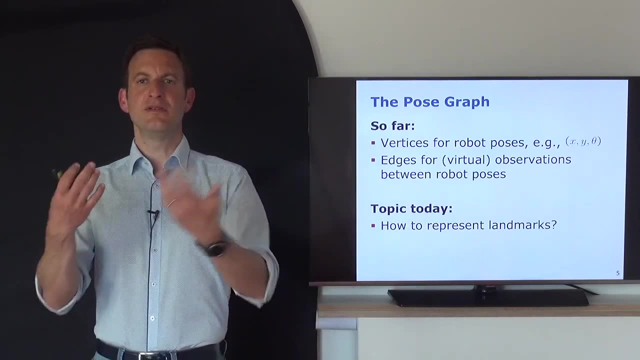 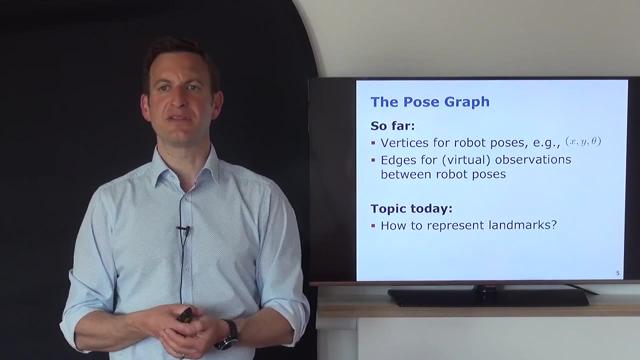 And in the postgraph we built the edges between those nodes through these virtual observations. So by observing the environment from two different places or two different points in time, and if you know that it is the same environment, we can say something about the relative transformation between the two recording positions, even if they happened at different points in time. 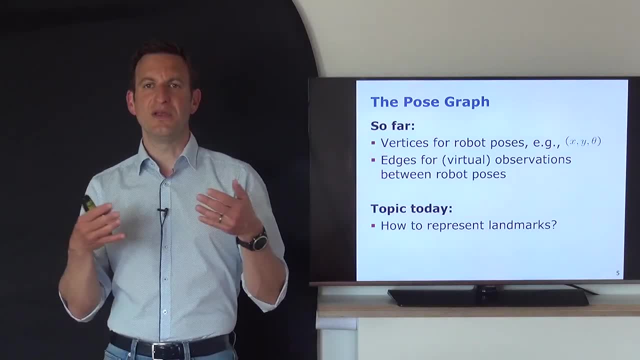 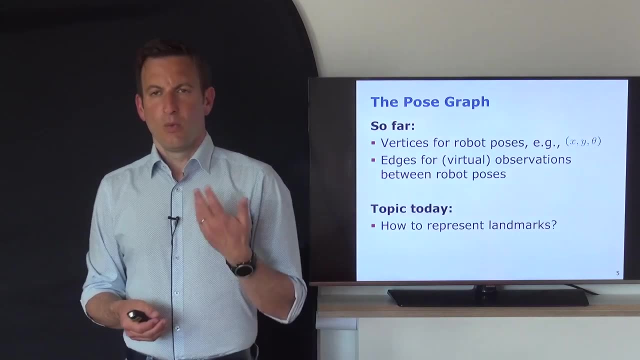 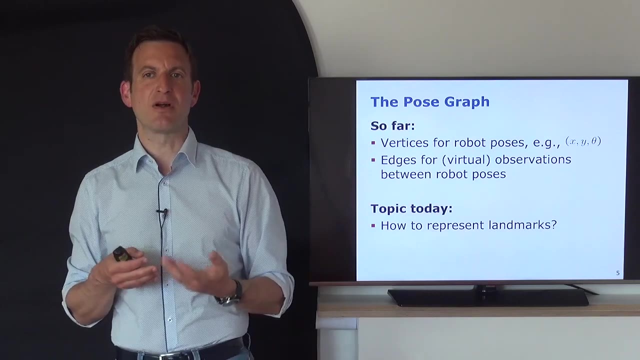 That was a postgraph and we now know how we optimize such a postgraph so that we get a minimum error configuration using the tools of least squares. What we're going to look into today is how can we do this if we don't have only post nodes. we also want to represent landmarks. 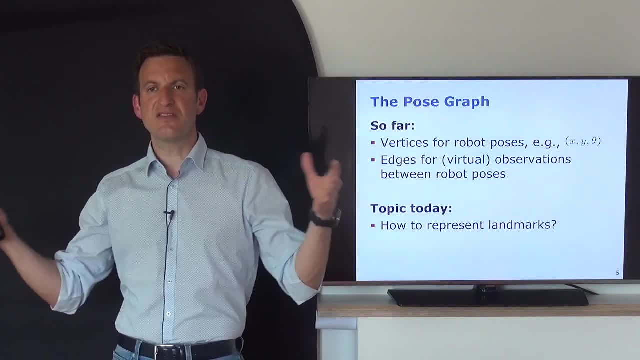 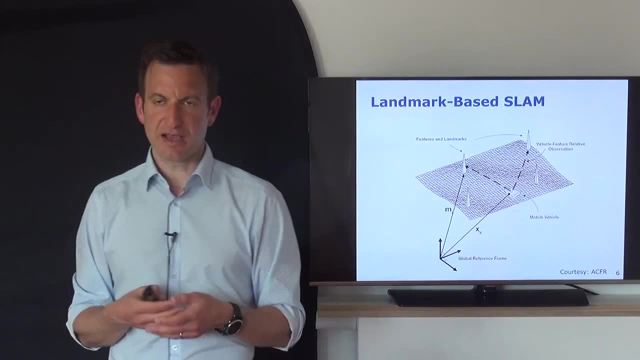 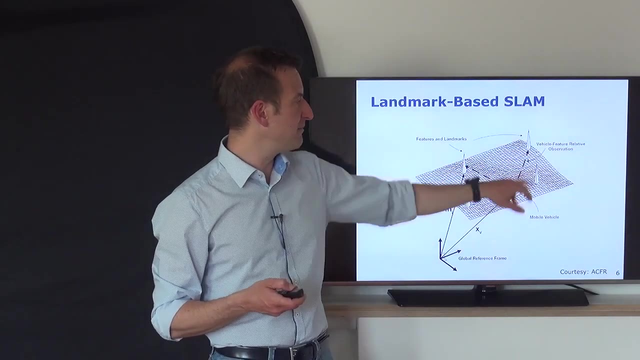 It means distinct points in the environment And we are not condensing this kind of local map information into this postgraph-like structure. So consider a landmark as some distinct point in the environment. So we have here this example of the mobile moving around and you have some landmarks or feature observations. 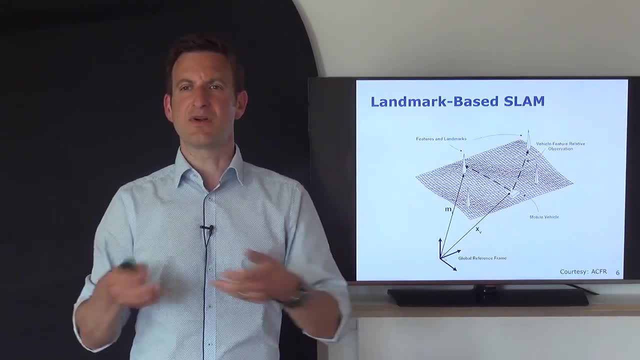 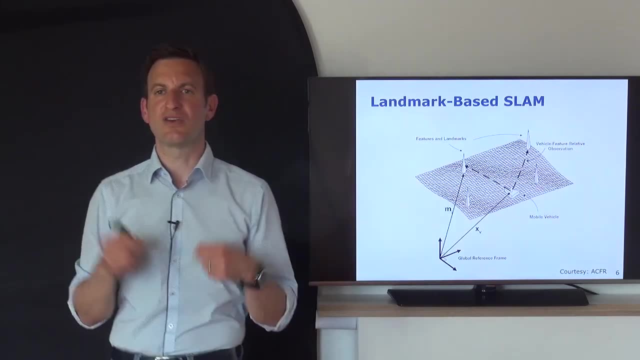 You can see this as lighthouses, as your landmarks, And you're on a boat driving in a bay and you can see the different lighthouses And you want to build a map to localize where those lighthouses are and estimate your own pose. 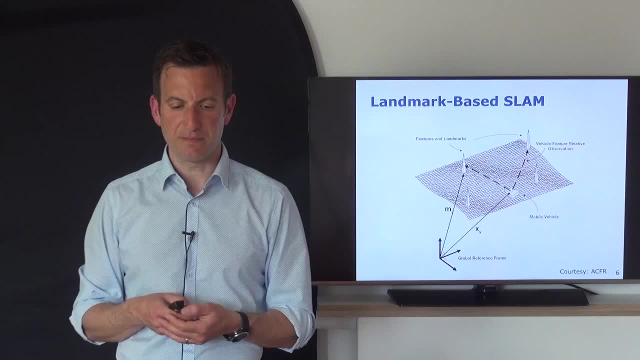 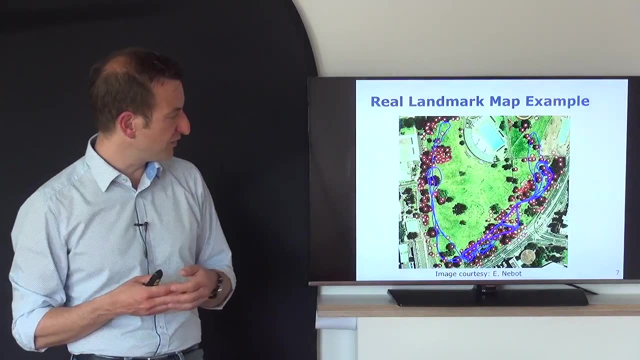 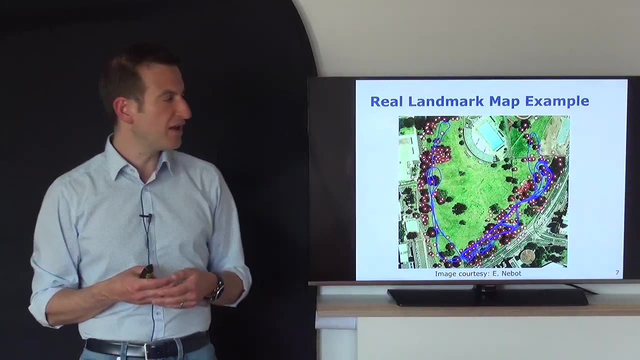 This is a traditional example for a landmark-based SLAM problem. You may not be on a boat. You can also do that by a vehicle driving through the environment. So what you see here is a. this is an aerial image of a very famous data set- Victoria Park data set recorded by the people at ACFR in Sydney several years back. 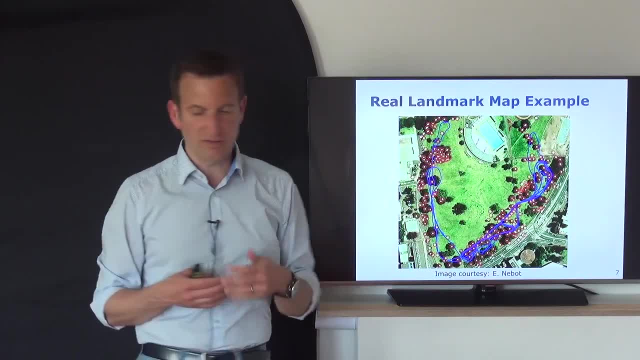 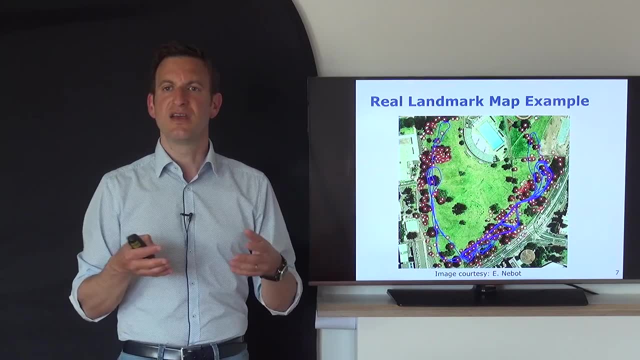 And in this data set you see a lot of trees in this park And there was a laser scanner mounted on a vehicle tracking or estimating the trunks of the trees, which served as landmarks or features generated from the scan, and every feature corresponded to a landmark tree. 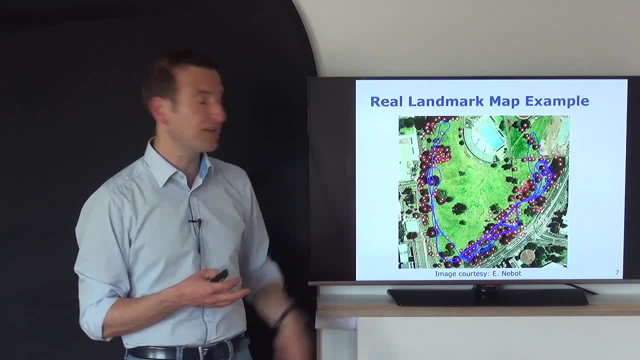 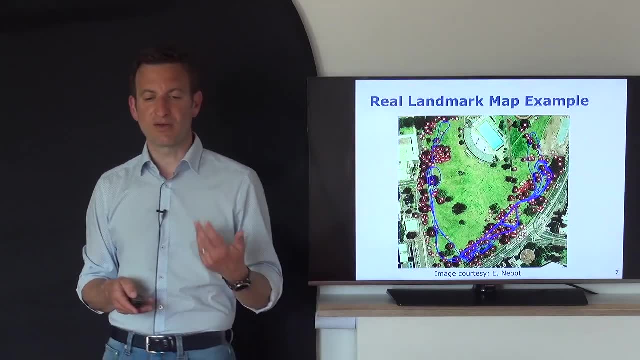 And then the task was to build a map of that environment, And this was one of the data sets which has traditionally been used in the context of an EKF-based SLAM, But of course it can also be used here for graph-based SLAM with landmarks. 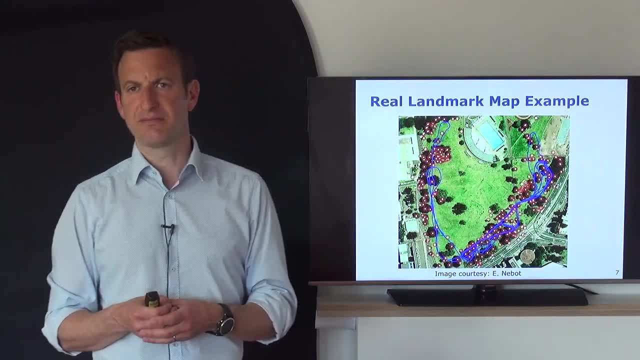 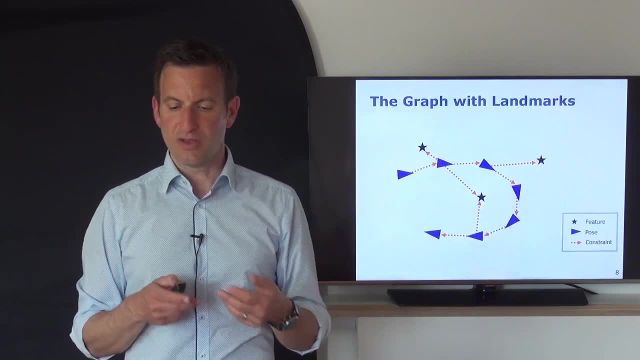 So what we can do now is we can add additional nodes to our graph And so that every of those landmarks, every of those tree trunks, becomes an own position in the map. So if we do this, in the idea of the graph-based SLAM not only having only poses, 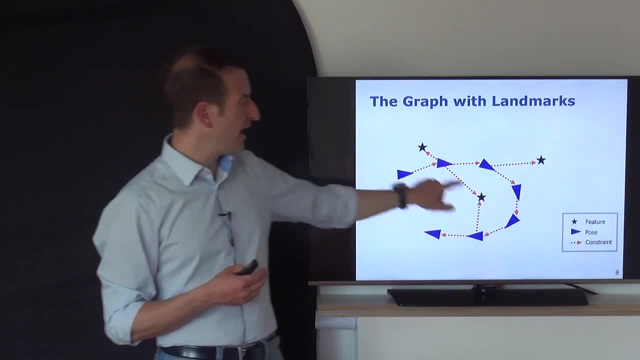 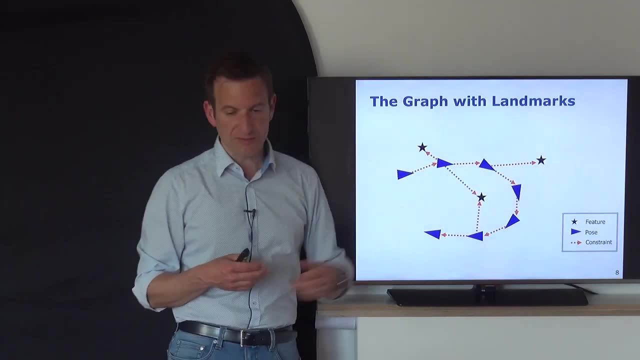 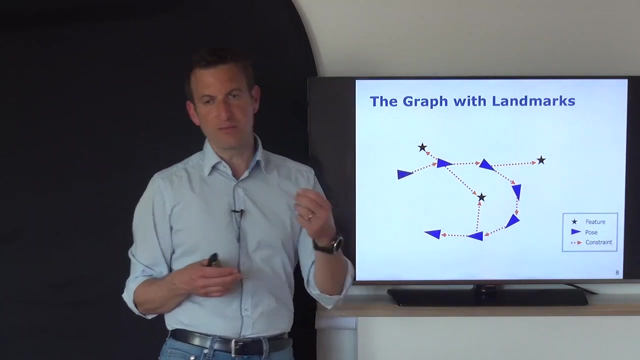 which is to be a position and an orientation, but we now have additional feature or landmark positions that we have, So this is given here by these black stars. So the difference now is that, while the robot poses typically as a position and heading information, 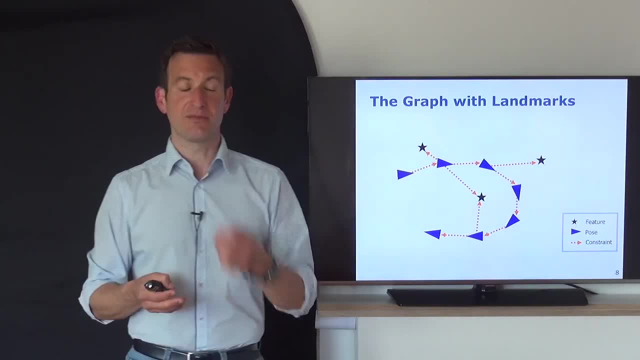 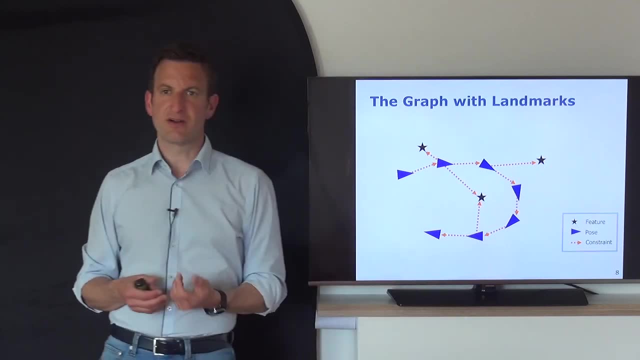 so x- y as a position and theta the orientation of the platform as a heading or, in 3D, corresponding x- y that your pitch roll. the position of the features in the environment are typically just positions. 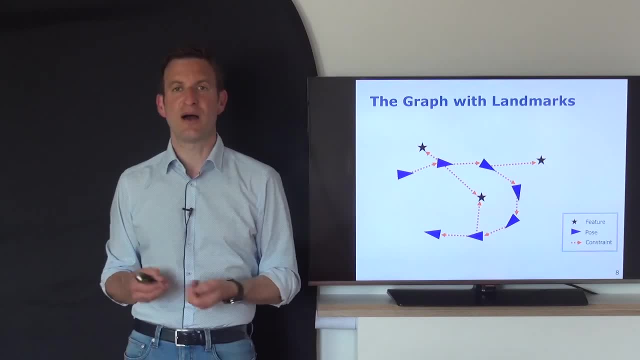 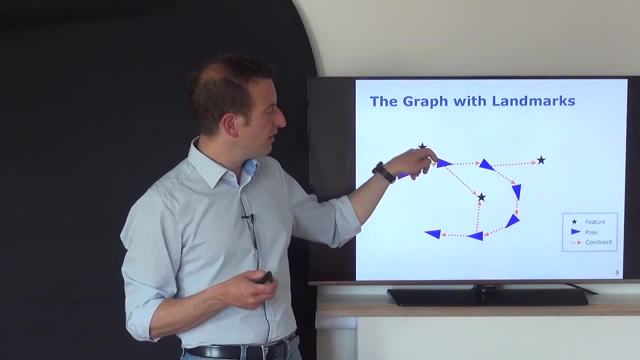 So they don't contain a position, Any orientation information, So it's just x, y or x, y, that, And so that's different, because then we don't have the full 3D transformations with position and orientation information between those edges. 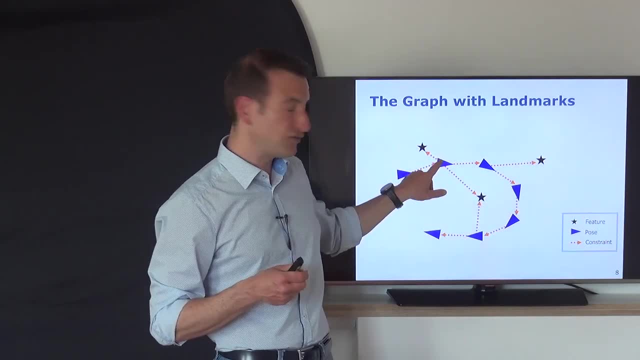 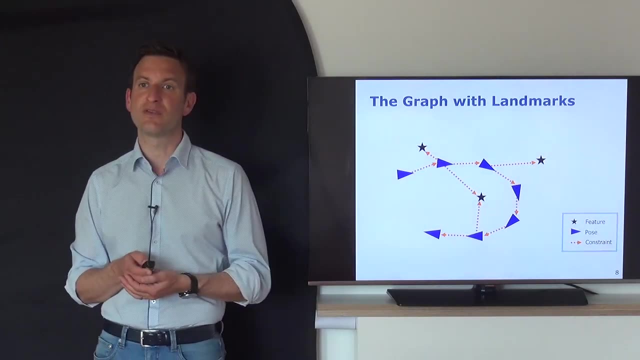 So the edges between the robot poses and the edges between a robot pose and landmark are different, And so we have different types of edges and different types of nodes now in our graph. So you can see this as a more complex graph: Different types of nodes and different types of edges. 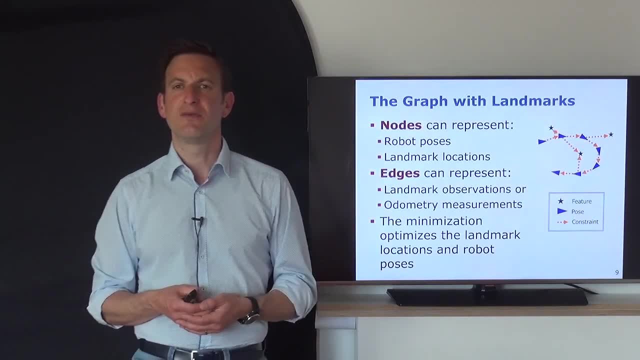 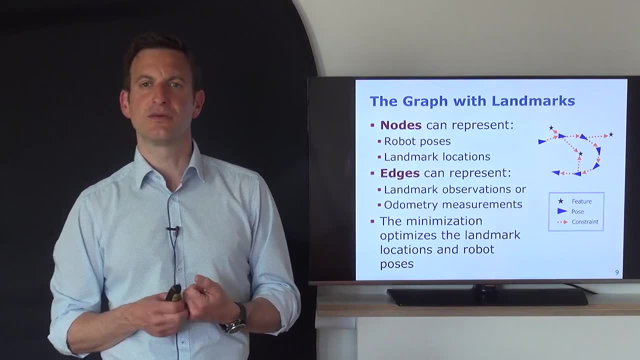 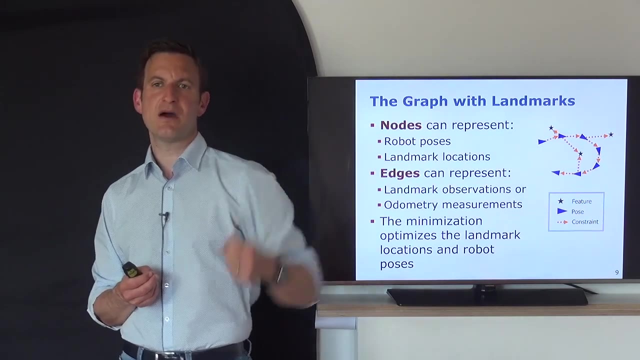 So in this landmark graph for the SLAM problem, nodes can now represent two things: Robot poses at different points in time and landmark locations. so positions And the edges between those nodes can be landmark observations. That means they connect a robot pose with a landmark. 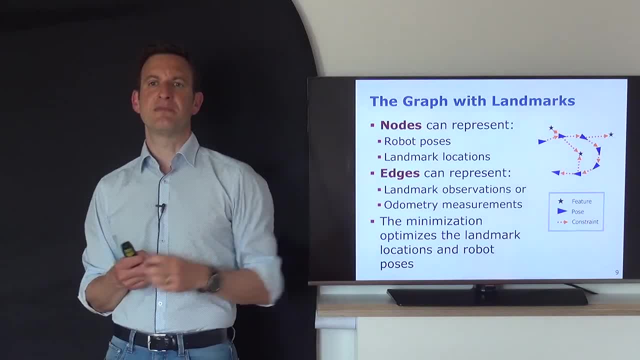 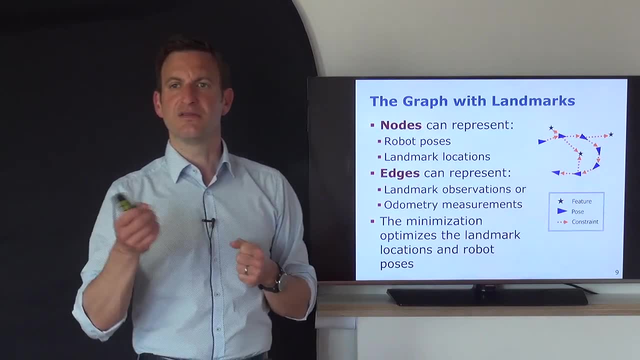 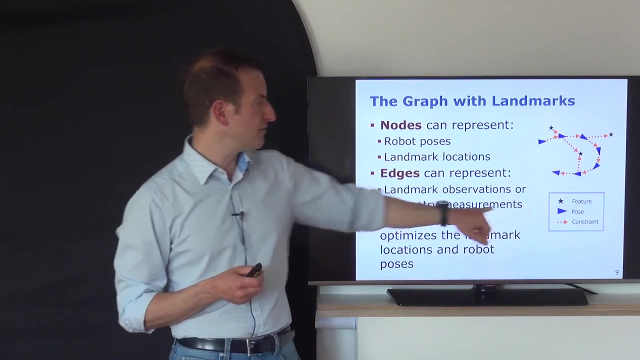 meaning the robot has seen a landmark from that pose. Or they can be odometry measurements. That means the traditional kind of consecutive links that we had already in our pose graph. So pose to pose constraint. So these odometry measurements are pose to pose constraints. 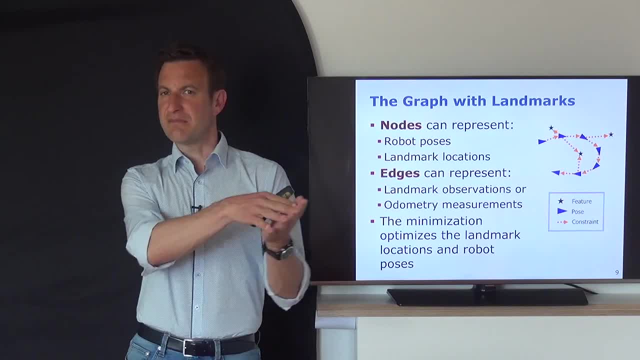 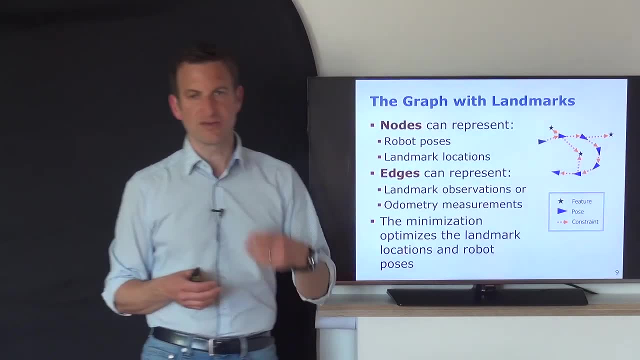 Could of course also be generated from scan matching of consecutive scans, if your sensor allows for this. But what we're interested here are those landmark locations, So the observations of the robot at a certain point, seeing a landmark somewhere in the environment. 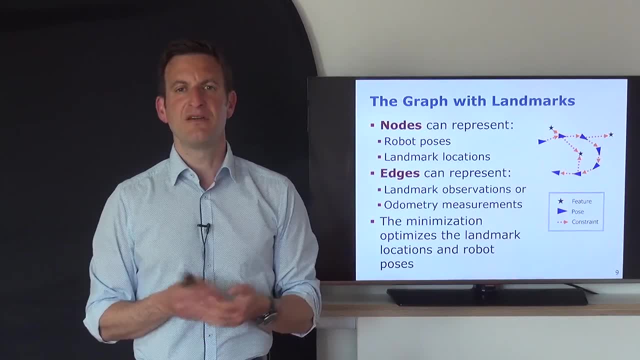 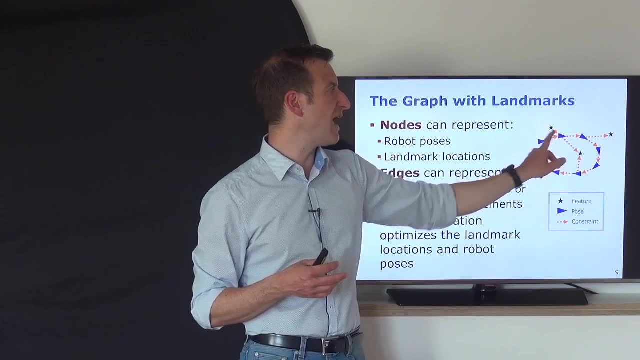 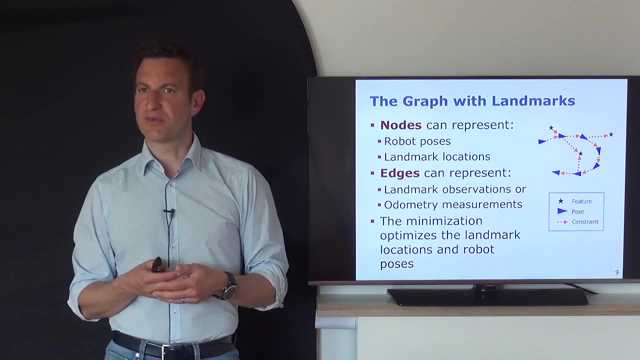 And again we can treat the minimization in graph-based SLAM very similar as we did it before. We want to find the new configuration of the nodes in the graph- And all the nodes are robot poses and landmark locations, So that the overall error is minimized. that results from the constraints. 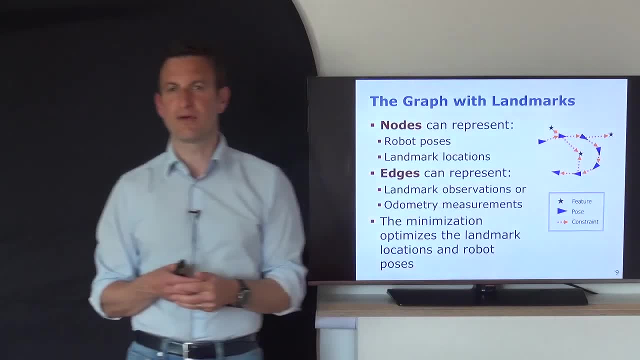 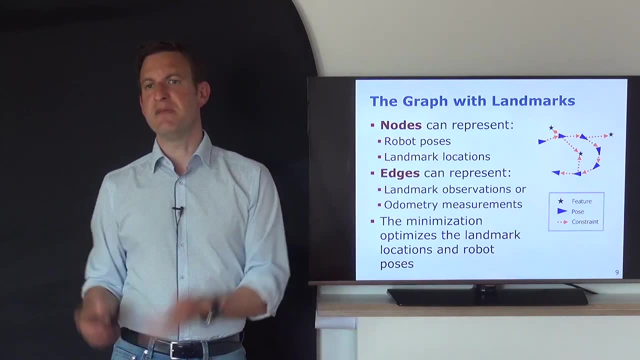 So the kind of error function that is associated to all of those constraints is again summed up: Square error is computed, And then we want to find the configuration of the nodes that minimizes the errors introduced By the edges or by the constraints. 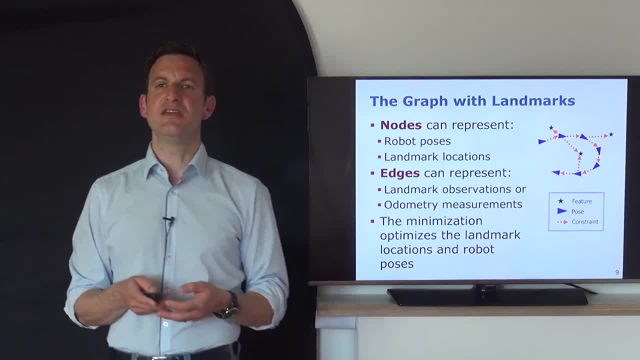 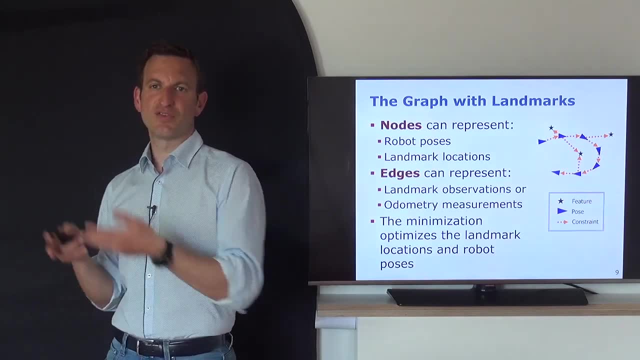 So it's a very similar overall idea. The main difference in here is that the graph structure now looks different, So we don't have the pose graph, It's only poses and pose to pose constraints. We have robot poses and landmarks as nodes. 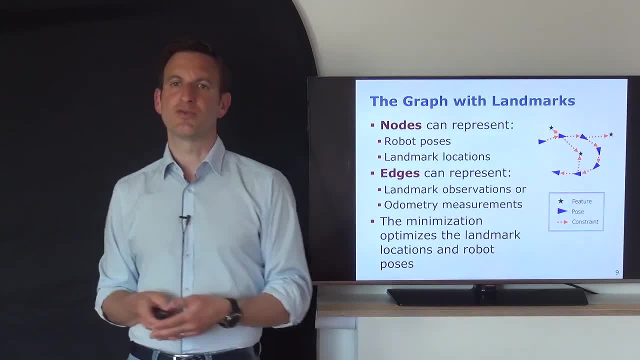 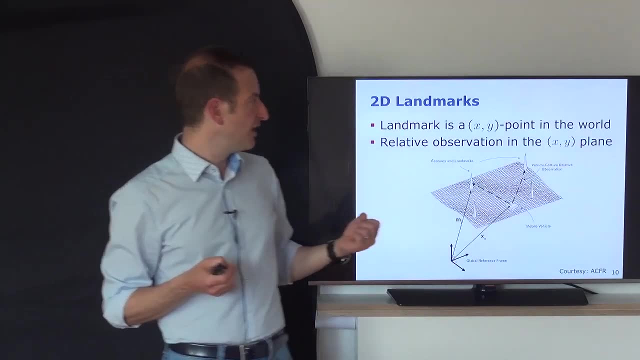 And robot landmark observations or pose, pose constraints, for example from odometry information. So, as an example, if you have 2D landmarks, the landmark can be 2D, XY point in the environment, two coordinates And the relative observation. 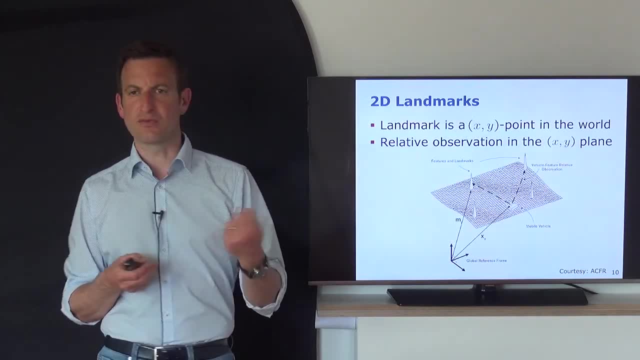 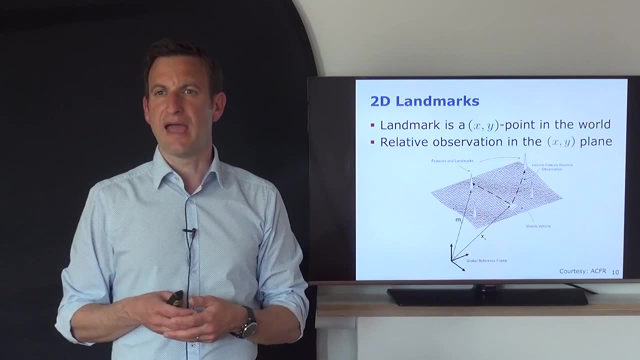 it can be the difference in the XY plane, It could be through a range in bearing observation, or it could be a sensor where this is converted already in a relative XY position. So delta X, delta Y from the current platform, given its heading. 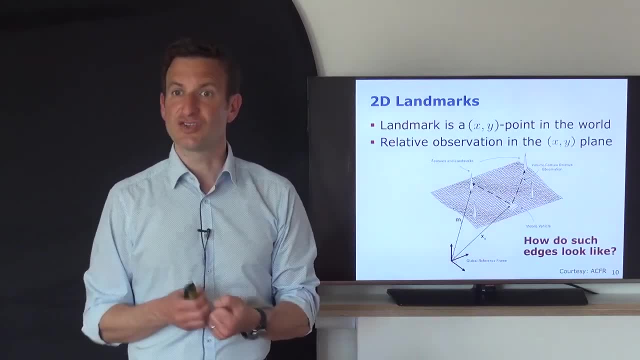 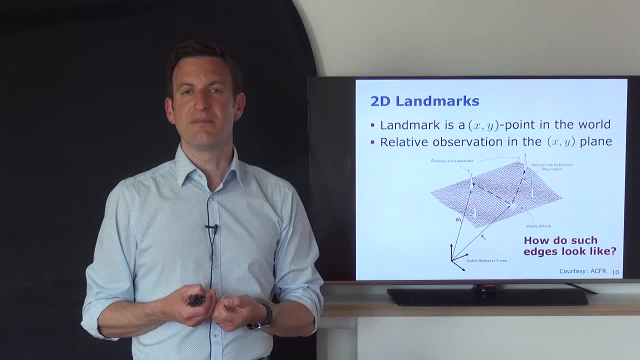 And so the key thing is now: how do such additional edges look like? That's something we haven't discussed so far. For the pose to pose constraints. we have the edges that we used in the pose- graph based SLAM, But now we have the additional edges. 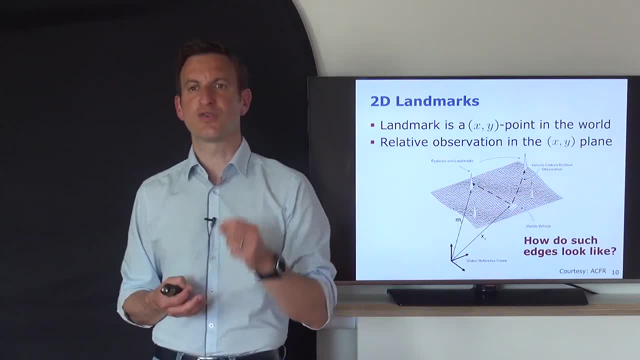 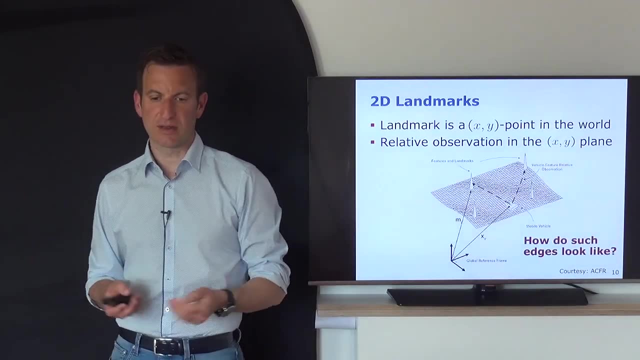 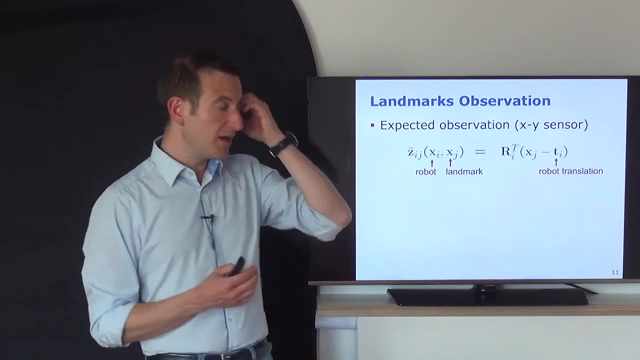 So in the next minutes I will just focus on how do those robot position or robot pose landmark constraints actually look like, Assuming here we have a so-called XY sensor which can measure the XY location of the platform, So similar to the pose graph based SLAM? 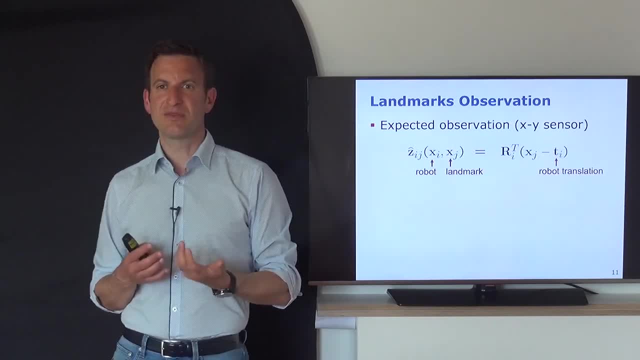 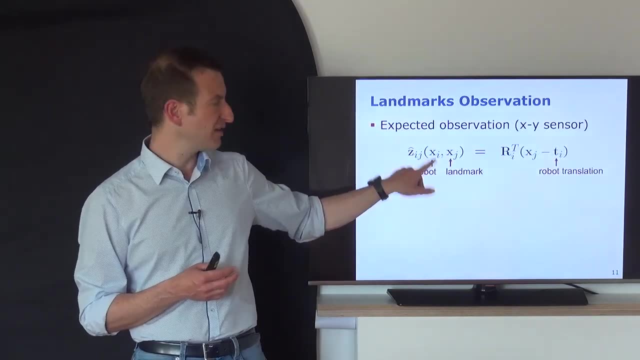 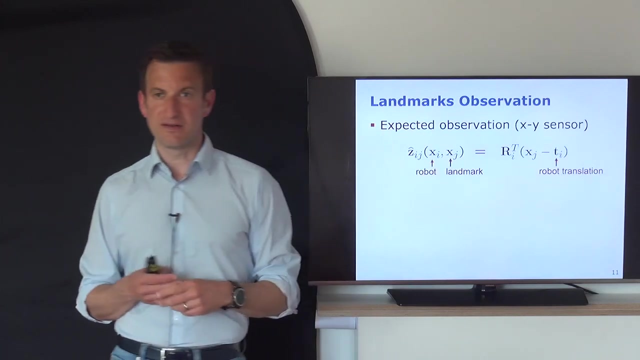 we have our expected observation And this expected observation obviously depends on where is the robot in the environment. So this is now an XY theta And the landmark location, which is now just an XY vector. So be aware that these are of different dimensions. 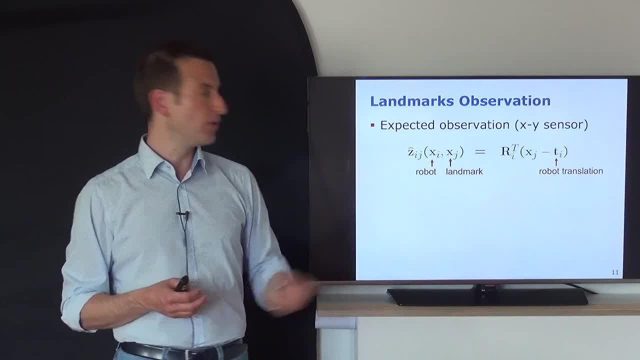 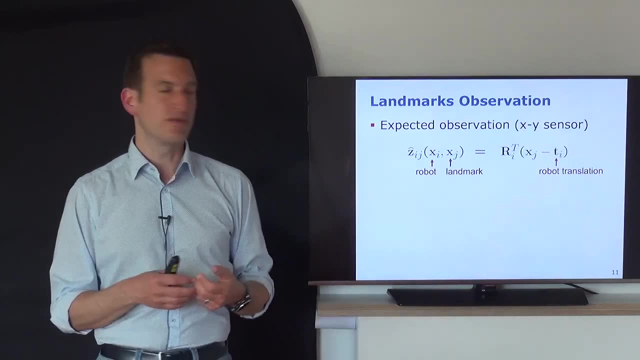 So the one is two-dimensional, the other one is three-dimensional, Or in the 3D world it would be six degrees of freedom worth of three degrees of freedom. And so how is one translated into the other? So we can say: this expected observation is basically given by taking the landmark location. 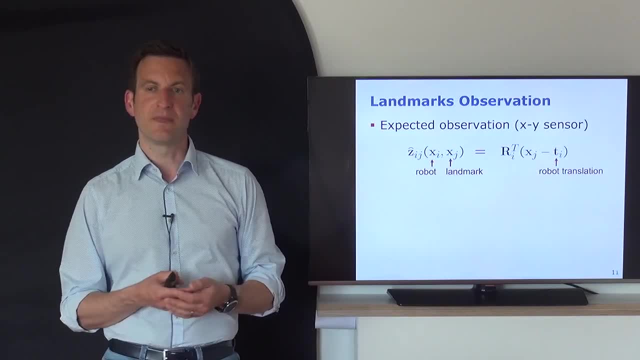 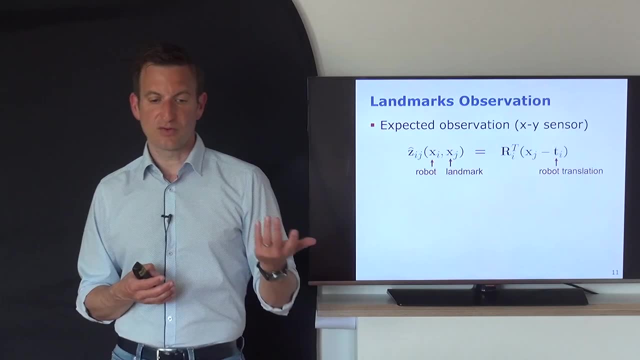 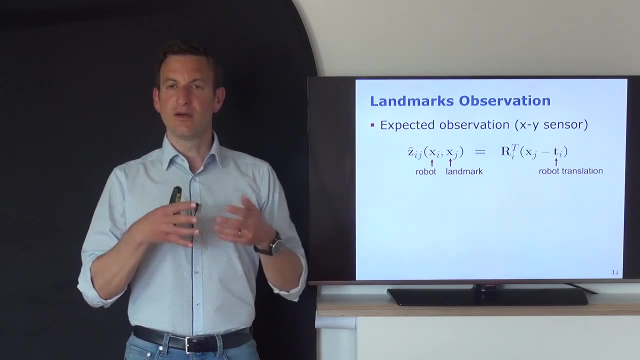 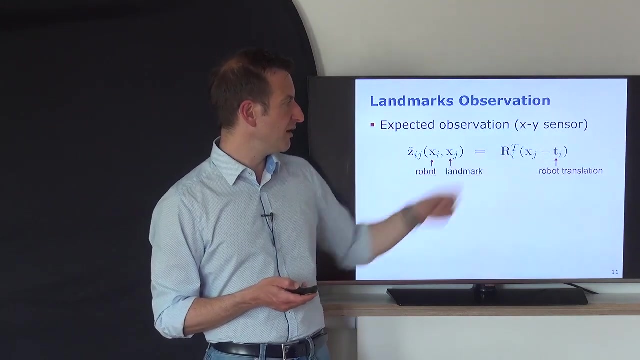 subtracting the translation vector of the robot location, so the XY coordinate of this part, and then multiplying it with the transpose of the rotation matrix encoding the orientation of the robot's pose, And this is a way to generate this virtual observation. So this virtual observation here would then be a 2D vector. 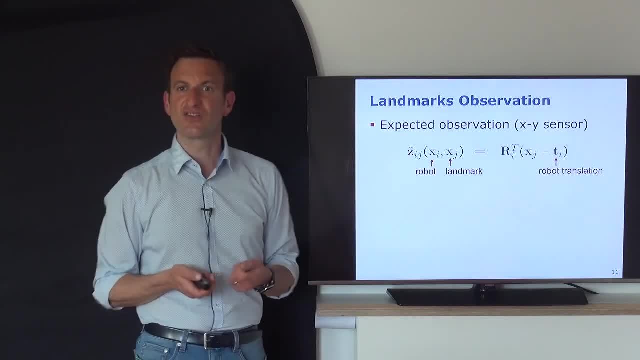 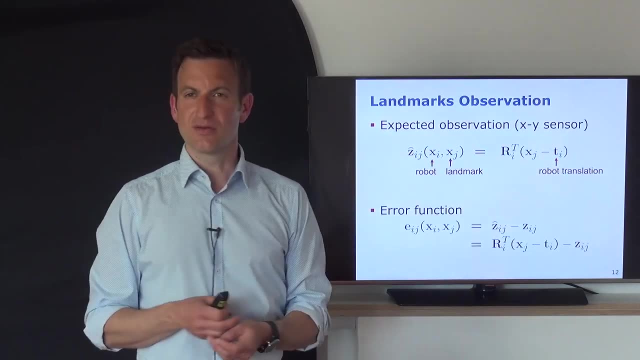 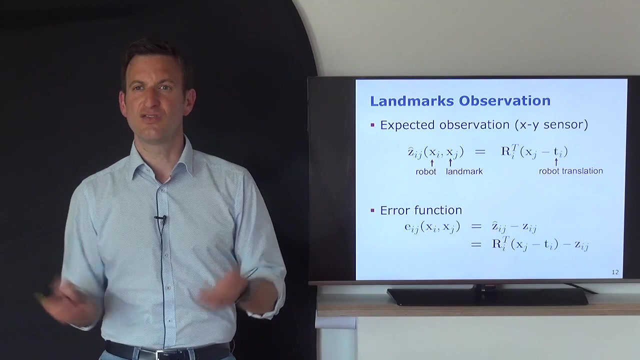 which is the outcome from that which is the expected X. So this is the Y observation that the platform should see. So relative XY location And this we can then use to directly derive the error function. So we can say my expected observation minus the actual observation that I obtained. 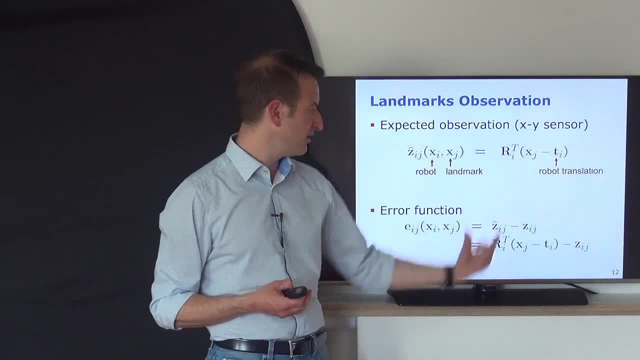 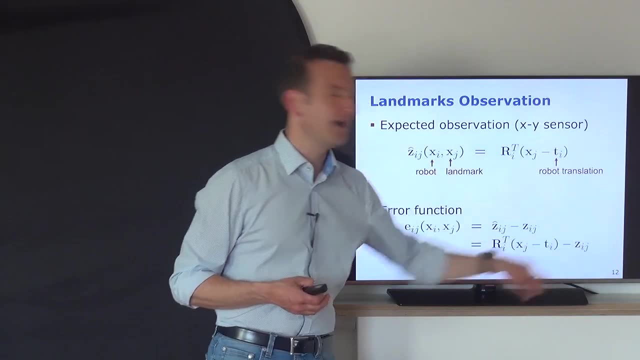 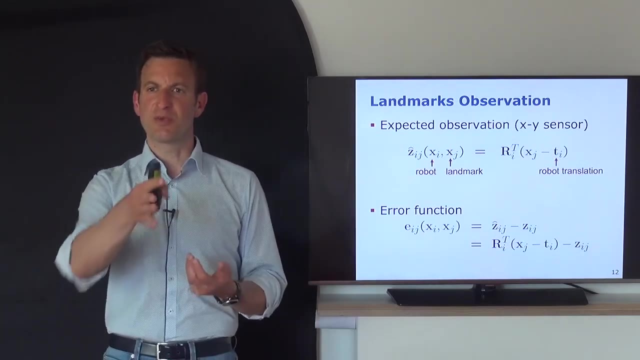 assuming I have this XY sensor And then we just take this equation over here, put it, replace it with Z hat IJ and put in this equation over here and subtract from this my actual observation, And that's it. So this is a very simple example for the simple case of having an XY sensor. 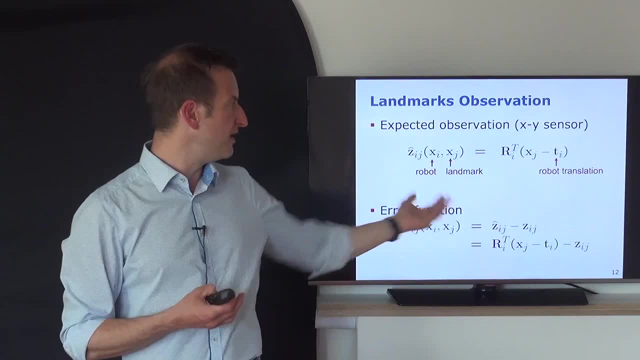 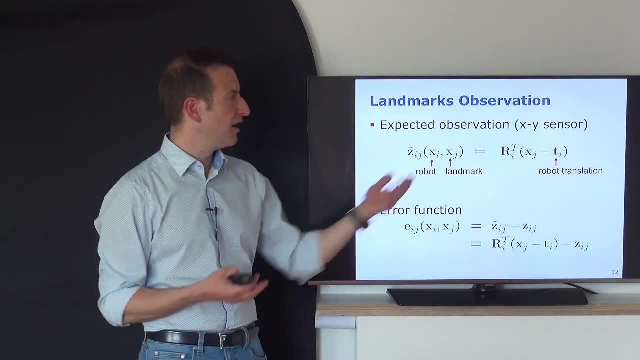 which tells me where the landmark is in a relative XY coordinate frame. given the robot's pose, This is how I can compute this observation, And obviously it depends on the sensor. Which sensor do I have? Do I have this type of XY sensor, yes or no? 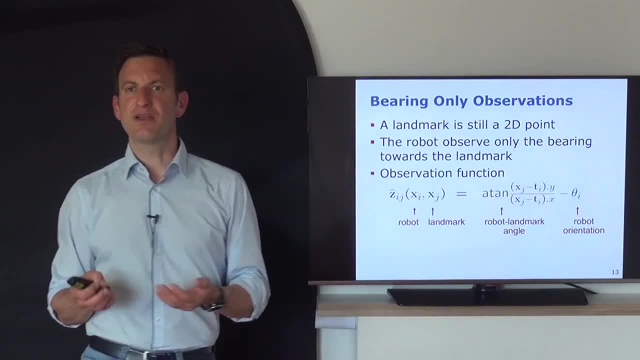 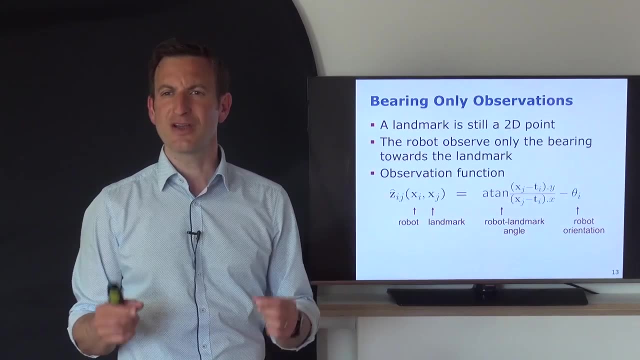 Another typical sensor that you may have, which provides actually less information than the XY sensor, is a bearing sensor which just tells you in which direction you can actually see a landmark. It's similar to a camera, just in 2D, where you can basically see, you just have an image. 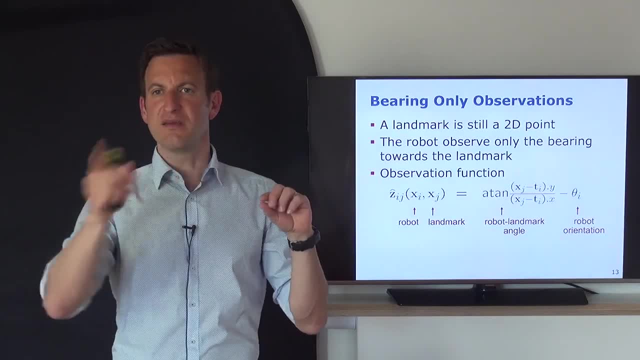 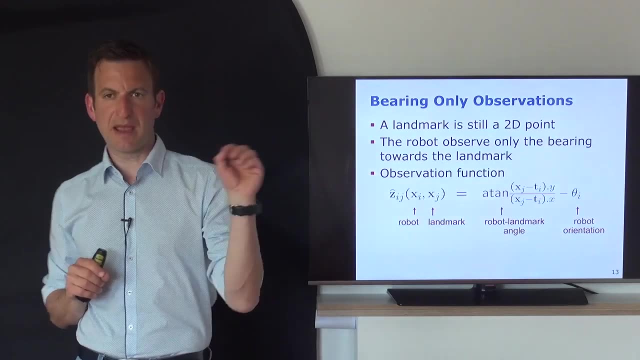 which just has one row and basically the pixel lights up where you see a landmark, in the kind of simplest case. So what you get is just a bearing, so just an angular observation that you have. So the landmark is still a 2D point in the environment. 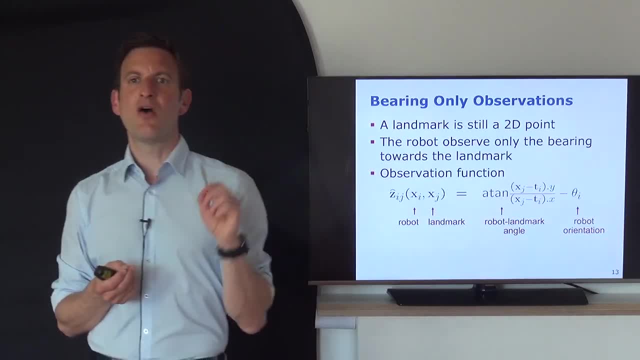 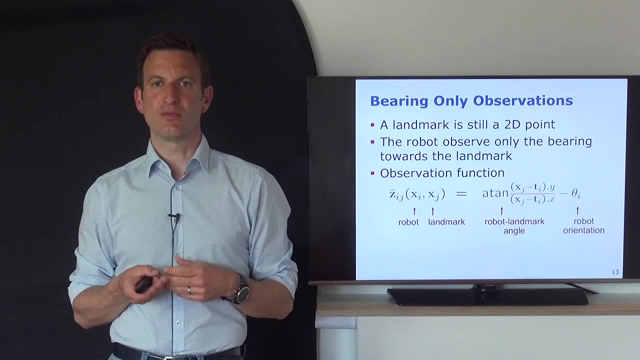 because it still is a point somewhere in space. but now my observation is just a 2D observation. Basically, what is the relative heading? Well, the relative heading of the landmark with respect to the robot. So, if I'm the robot, I'm looking forward. 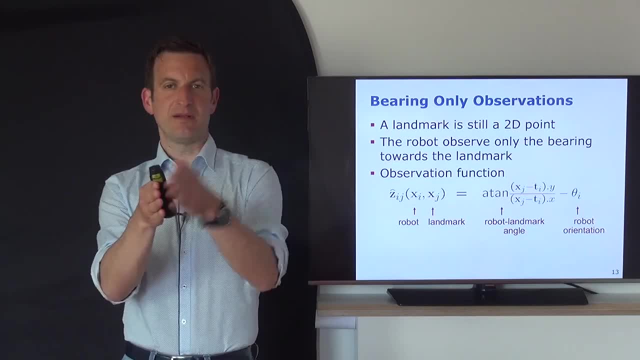 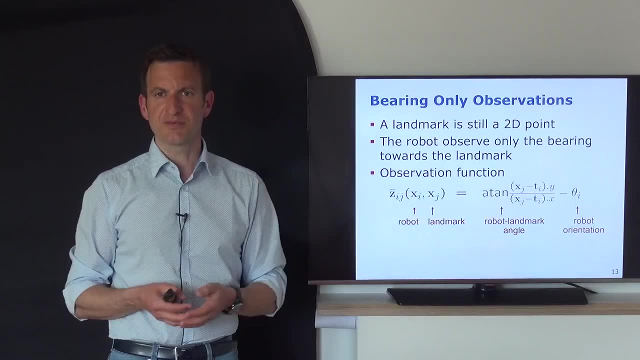 then a landmark being directly in front of me would give me an observation of zero. If I would, for example, be 10 degrees to the left, then I would get 10 degree as my observation. We compute our predicted observation in order to estimate what the robot should see. 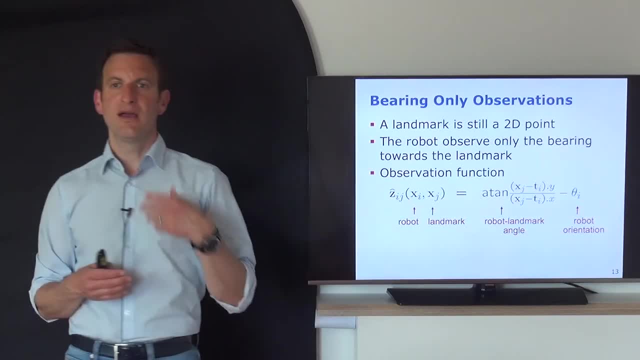 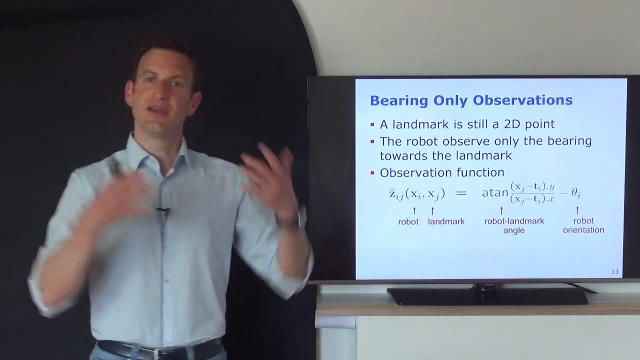 We need to know where the robot is and where it's looking to, which is again stored here in Xi, And we need to know where this 2D landmark is in the environment. So we can compute this by looking to the difference in the y-coordinate. 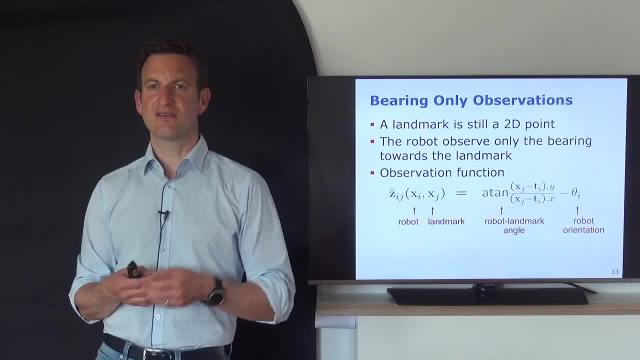 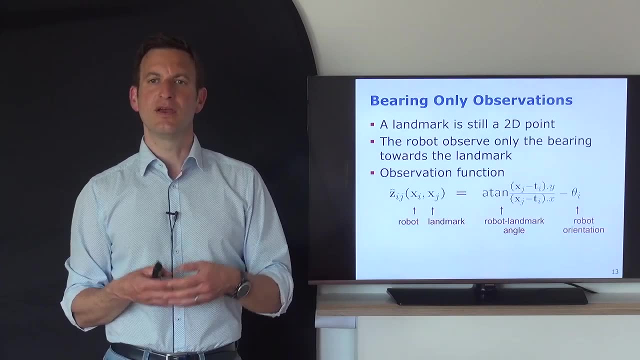 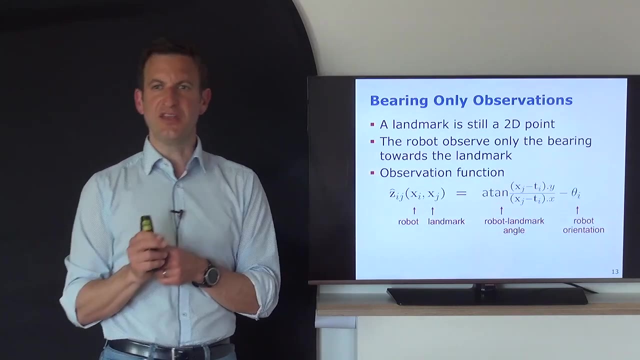 minus the vector vector shown over here, exactly the same as previously in the Xi sensor. The only difference is that this function that had is now a one-dimensional function, not a two-dimensional function. So it has a 1D output just providing the angular component and not xy or delta xy as it was before. 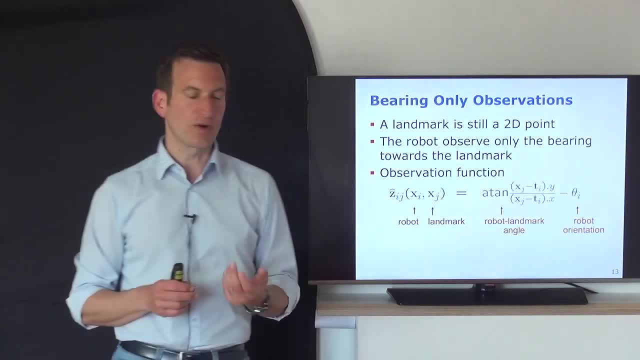 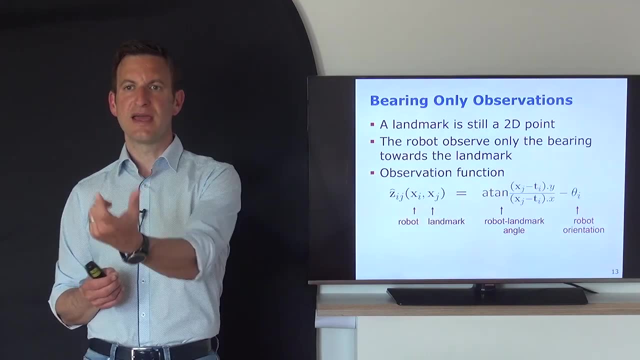 So how do we compute where the robot is and where it sees the landmark? Well, we need to know the x-coordinate and the difference in the x-coordinate between the robot's location and the landmark, which is here given by xj minus ti. 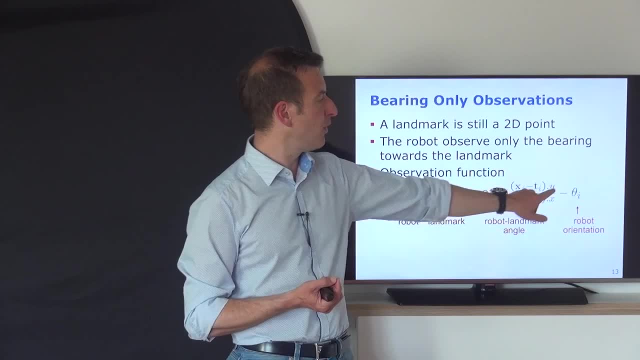 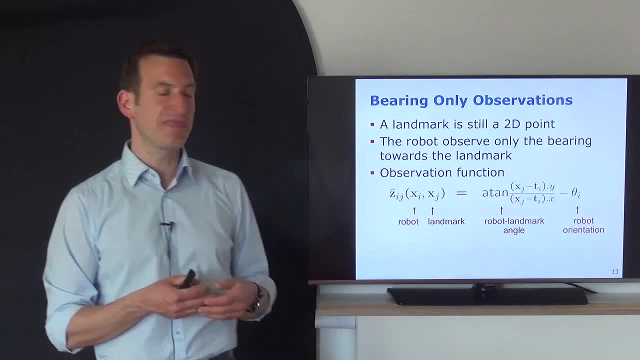 So this is again the transformation vector or translation vector resulting from the robot's pose. We are just taking the y-coordinate into account and the x-coordinate and computing the aton of that. So if you implement this, you would use of course, the aton2 function in order to do this. 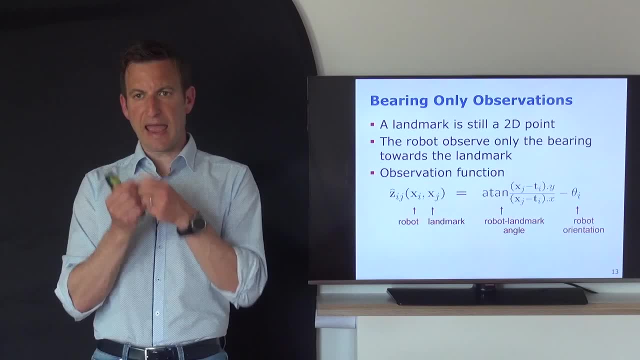 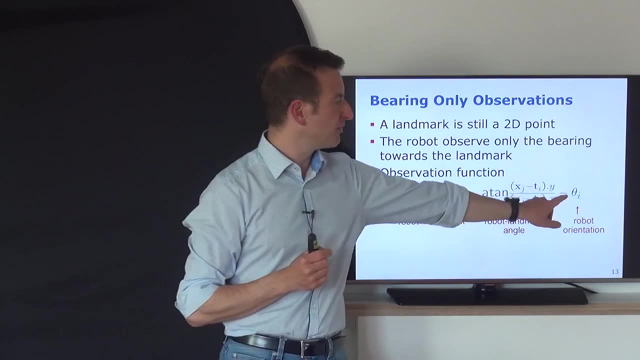 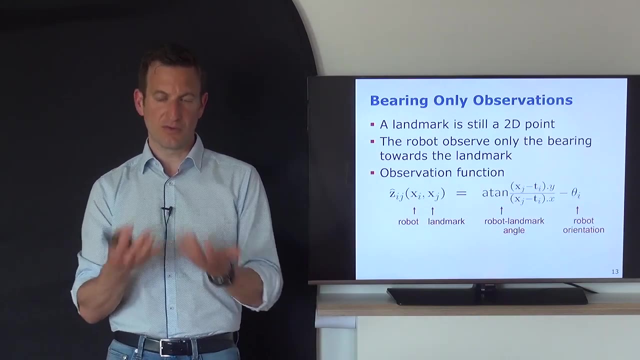 in order to have all the quadrants done right, which is the angle between the robot's pose with respect to the landmark in the global reference frame, And what we need to subtract from this is the orientation of the robot, because there's obviously an observation which is done relative to the robot's current heading. 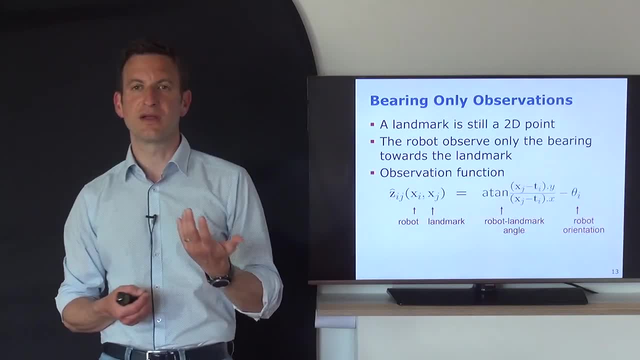 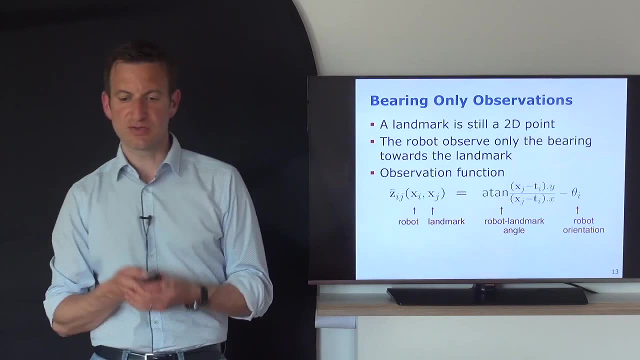 So this is basically in the global coordinate frame and this turns it into the local coordinate frame, because we need to see it as the robot would see it. So this is my expected observation function, or my observation function which computes me. So this is my expected observation and from this I can then directly derive the error function. 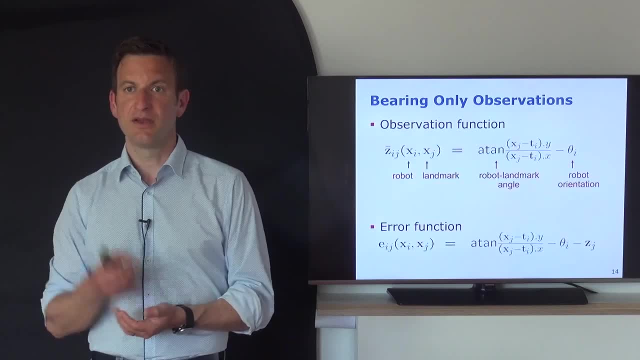 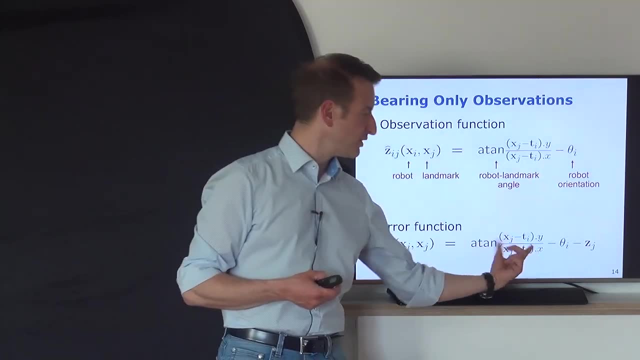 because the error function was just the predicted measurement minus the actual measurement. So this is then, straightforward: My error function for that bearing-only observation is what I'm predicting to see, which is this part over here minus what I'm actually seeing. 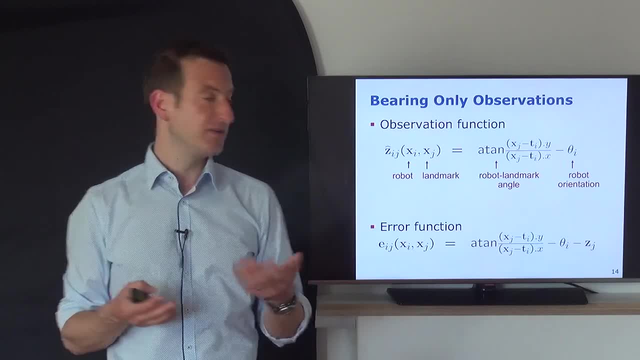 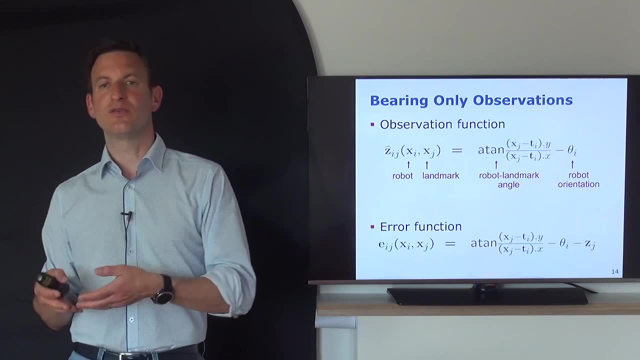 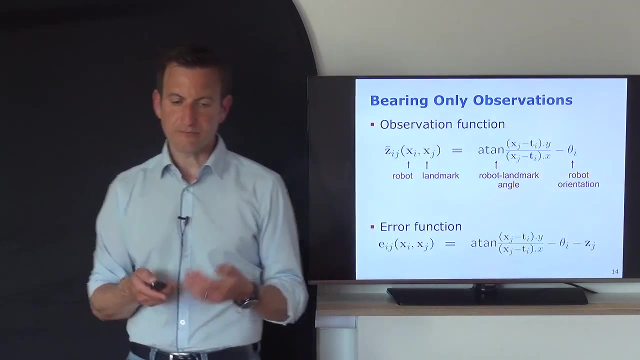 So what was the observation of this landmark j? And again, this is a 1D function. in this case, The xy-sensor was a 2D function And compared to the post-graph observation into d, which was a 3D function that we get out of here. 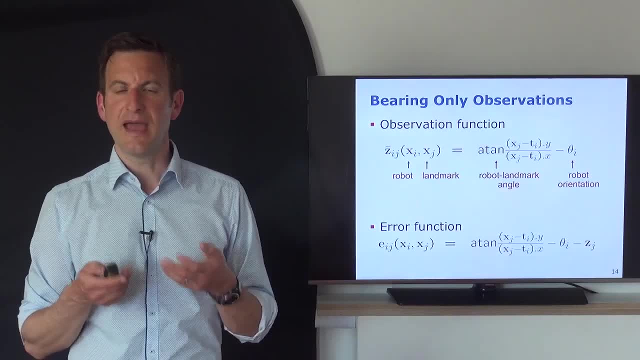 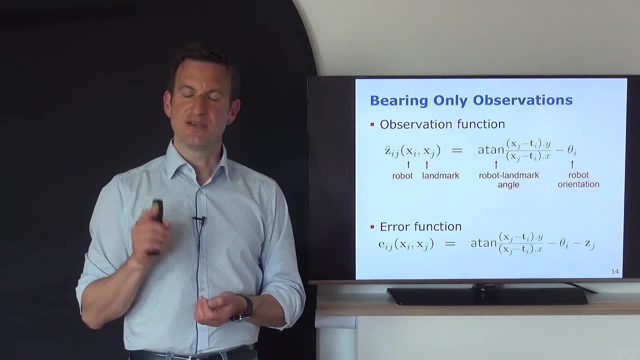 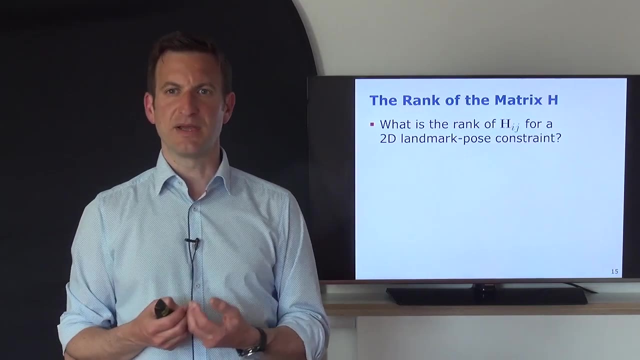 And this actually impacts the h-matrix that we generate for this observation. Again, this was computed by having the Jacobian transposed times the information matrix, times the Jacobian. This gives me the element for this h-matrix. So we need to look a little bit into the rank of this h-matrix. 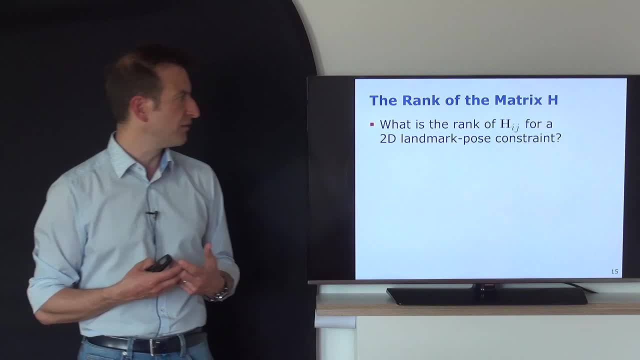 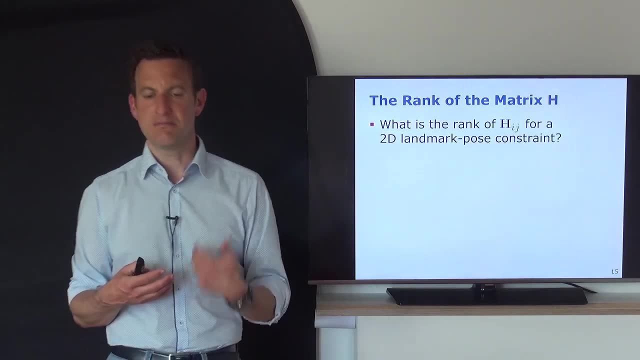 because this turns out to become important or is an important information. So the question is: what is the rank of this h-matrix? So the question is: what is the rank of this h-matrix for the 2D landmark post-constraint? 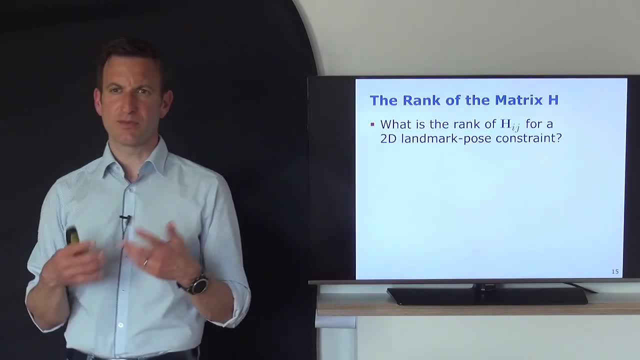 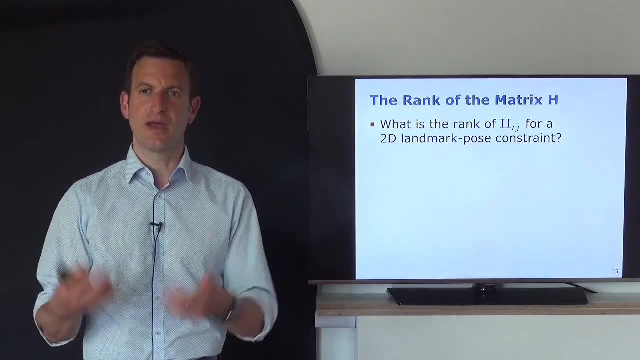 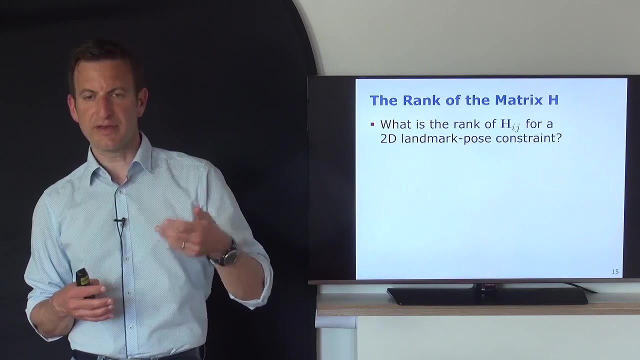 If we have a matrix, let's say A transpose A- and we want to compute the rank of this matrix- A transpose A- then this rank is equal to the rank of A transpose and the rank of A. And this is important because this matrix H is built up by taking the Jacobian transposed times, the Jacobian. 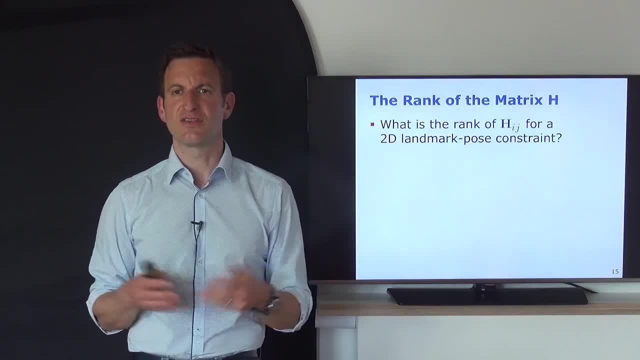 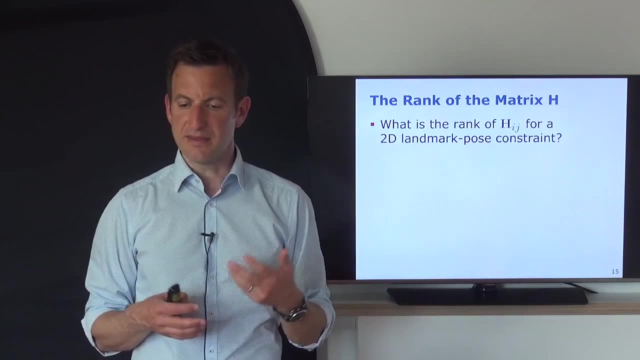 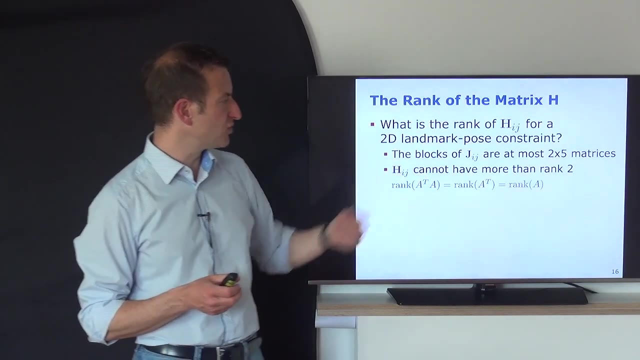 Of course with the information matrix in between. but assuming the information matrix itself has full rank, then the rank of this h-matrix is basically determined by the rank of your Jacobian. And if you look to the blocks of this Jacobian, 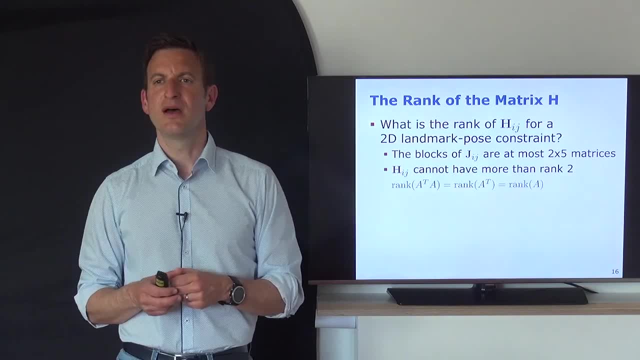 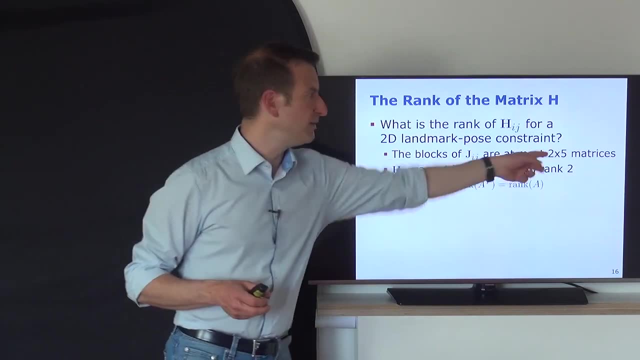 this is at most a 2 by 5 matrix, which is non-zero. So 5 for the parameters x- y- theta of the robot and x- y of the landmark, And 2D because it provides you 2D information. 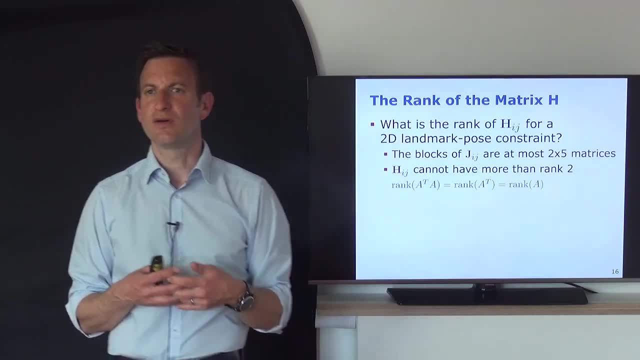 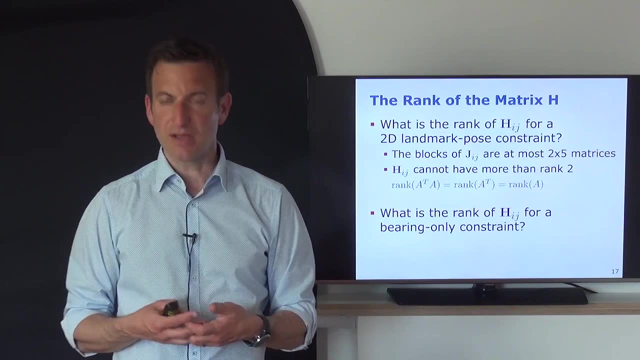 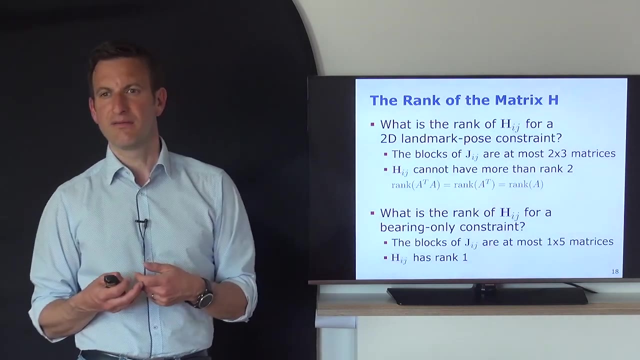 So hij can't have a rank more than 2.. So at maximum you can kind of fix 2 degrees of freedom in here. And if you look to the bearing-only constraint and compute the h-matrix, then, even more extreme, you have a 1 by 5 matrix. 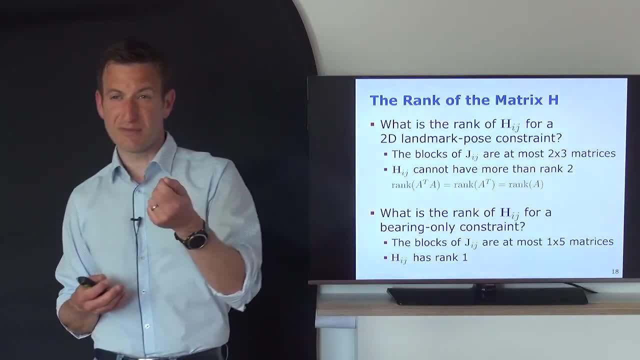 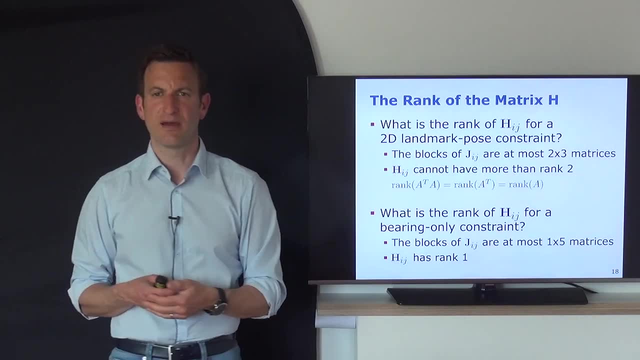 So because you have 1 degree of freedom for the measurement and 5 non-zero elements for x- y, theta and of the robot and x- y of the platform, So hij, in this case only have a rank of 1.. 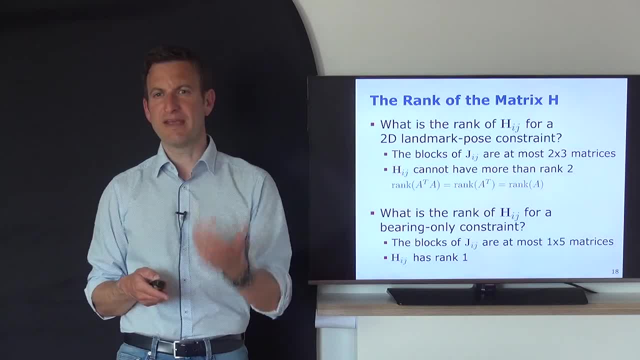 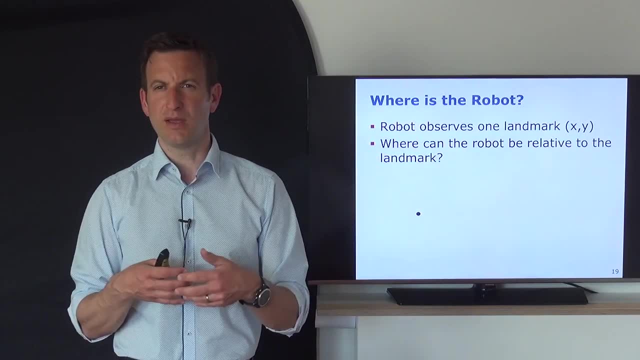 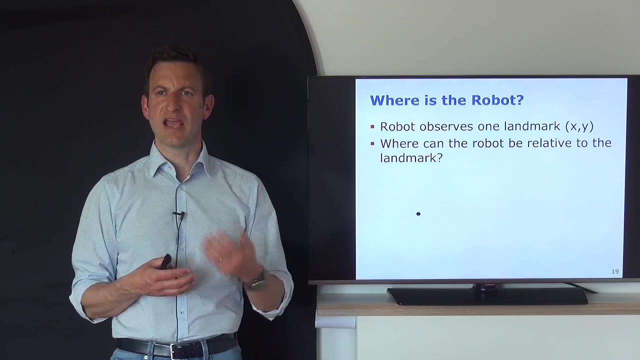 And this has an impact on what information such a measurement can provide. And I want to show this with a small example saying: where is the robot? assuming we know where the landmark is and want to now localize the robot. And let's see for the first example that it is an x- y observation. 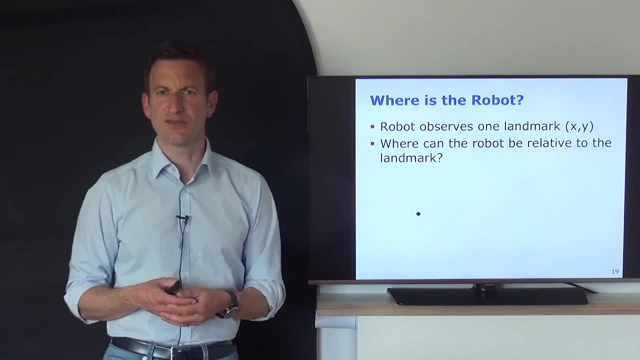 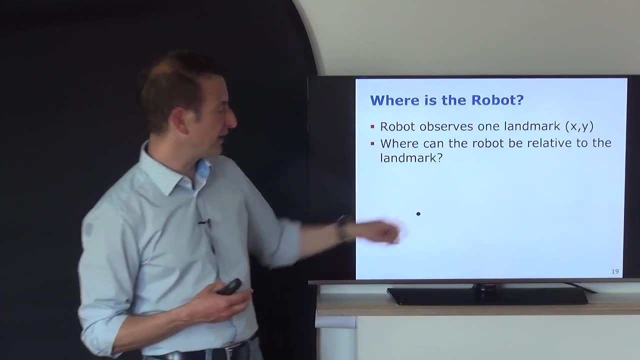 So the robot observes an x y landmark and we have this relative x y sensor. So if you have one single observation, where can the robot be relative to that landmark? So assuming this black dot here is a landmark, and assume we have a delta x, delta y sensor, 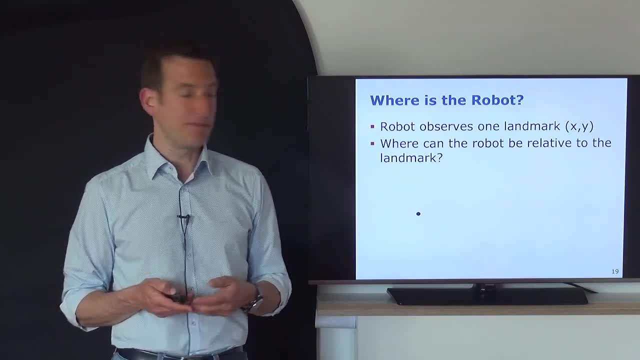 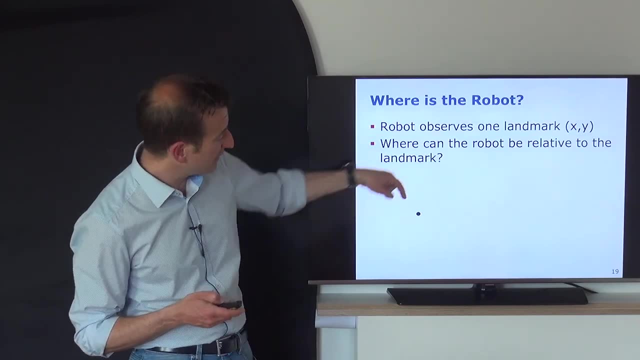 So where can the robot actually be in the x- y plane? And it turns out that the robot can actually be at multiple places and would get the same observation. So the robot can basically be arranged in a circle around that landmark And the position of the circle then determines where the robot is actually looking to. 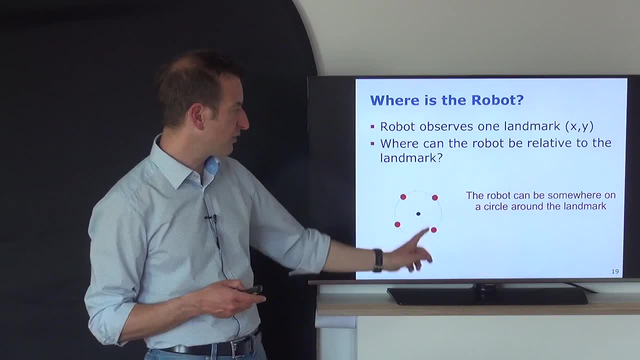 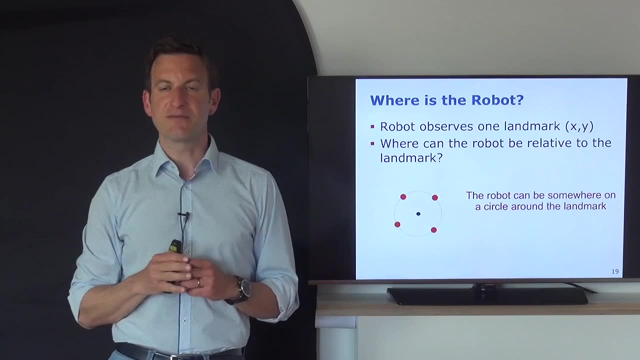 And it will look like this. So the robot can be anywhere on that circle. And if I fix the position of the circle, it will tell me where the robot should look to. So, for example, if the landmark is directly in front of me. 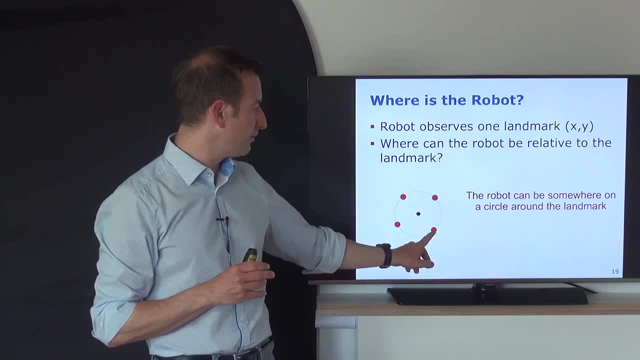 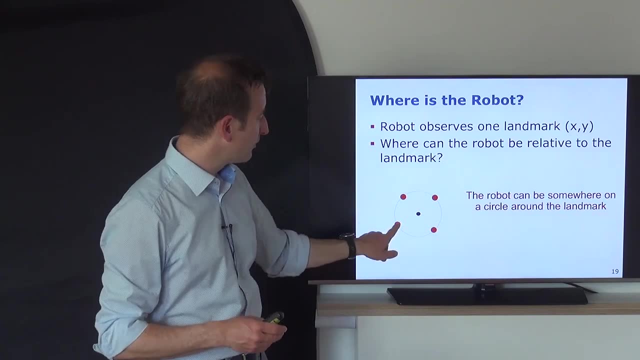 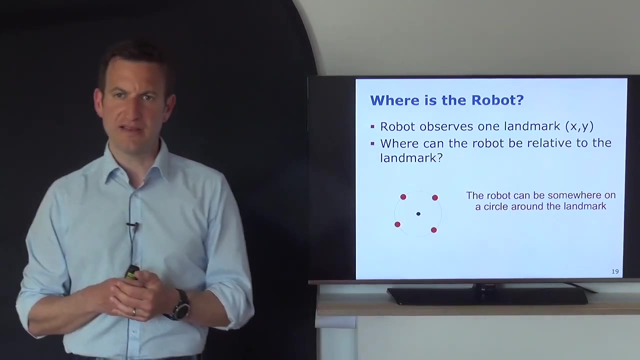 then all these positions here, the red possible positions, will point directly towards this landmark. If the landmark is right of me, this robot would look in this direction. this robot would look in this direction. So this rank two constraint allows me to fix two of the three parameters. 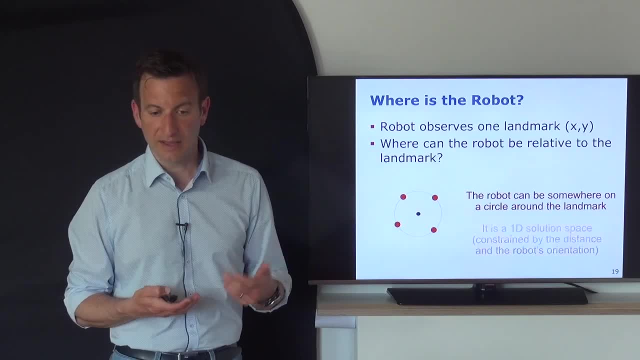 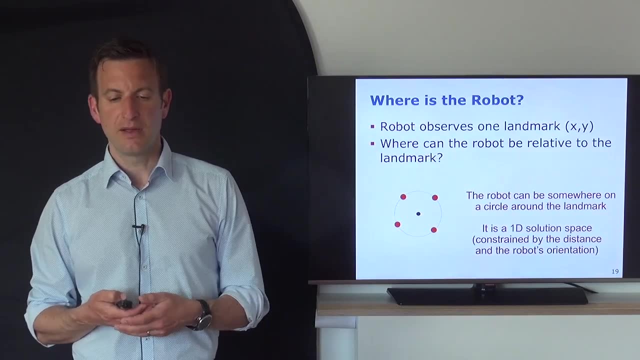 that determines my robot location. Right, So I can be anywhere on that circle. It's a 1D solution space And the orientation is determined by where I am on that circle. And now we can look. how does it look like? if we have a bearing, only observation. 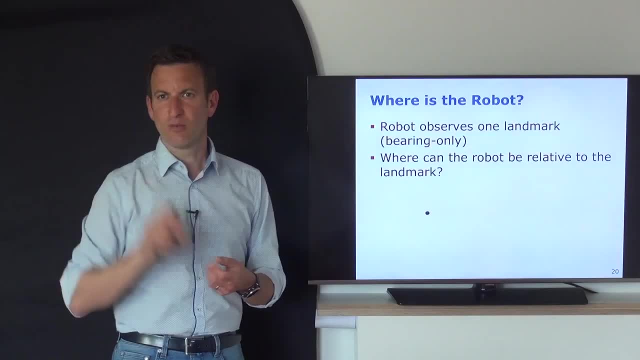 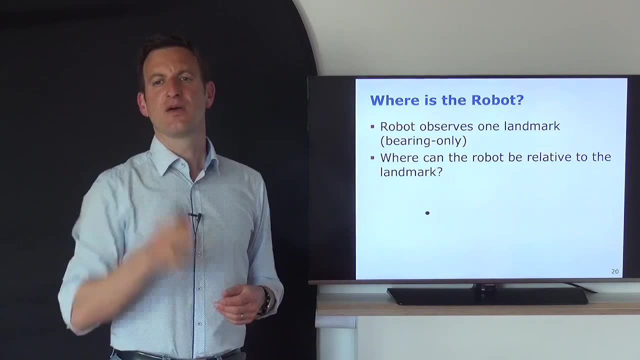 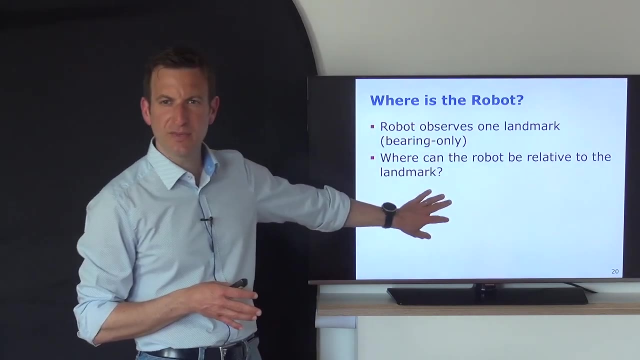 So exactly the same setup, but now we only have one direction we look into. So this is our landmark location And I just know where the robots see the landmark relative to each other in terms of one rotational angle, In this case the landmark- the robot can actually be anywhere in the 2D space. 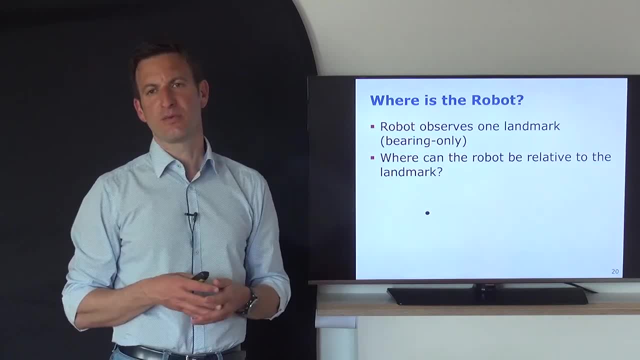 And depending on the position of the 2D space, we are actually fixing where the robot is looking to. So again, if you think the landmark is directly in front of the robot, but you have no idea how far it is away, 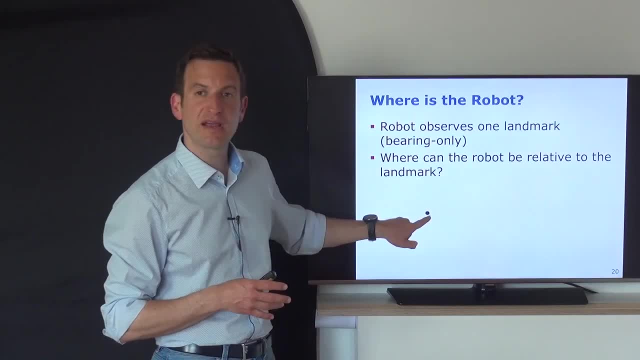 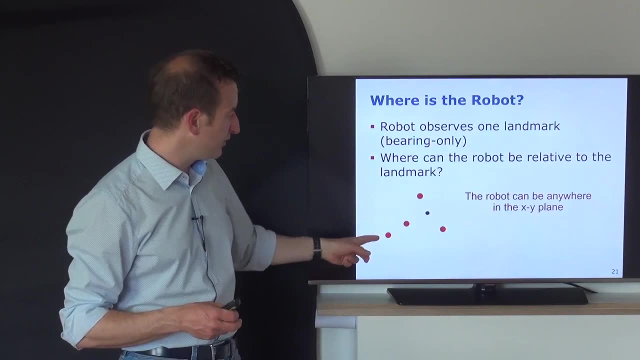 the robot can be anywhere in the space And wherever it is, it will point directly to the landmark. So, sitting here, the robot will be looking here. If the robot is here, it will be looking over here. So just as a few examples, these are possible locations. 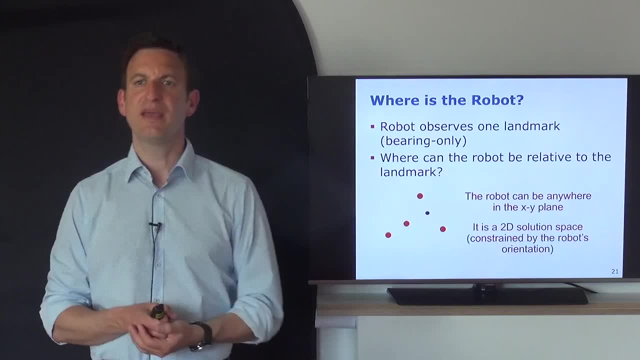 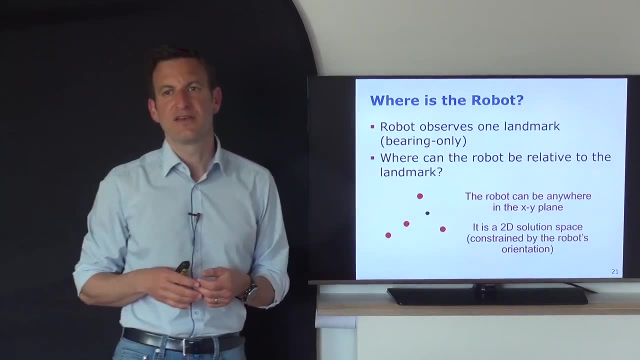 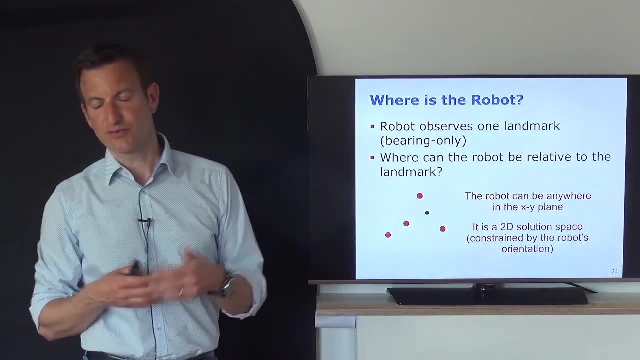 and all the robots would look towards this landmark. So any space, any position in the XY plane is possible, And if you select the position, then we actually fix the orientation of that platform. And so in this example, the rank of this constraint is one. 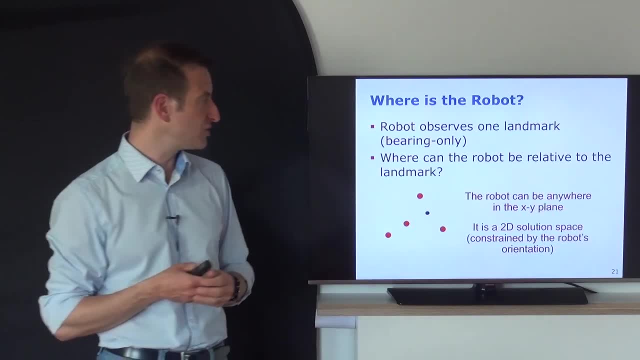 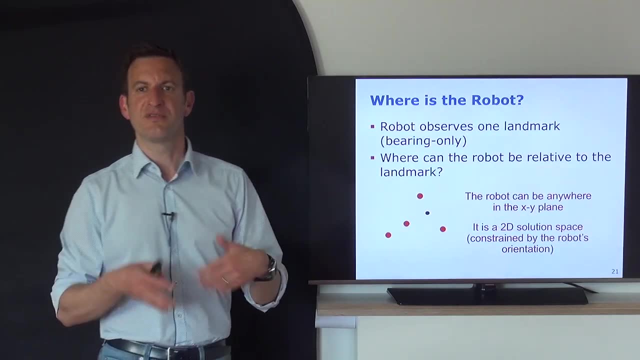 I guess we had the one dimension of the Jacobian is just one dimensional, So rank one. we have three degrees of freedom that we need to fix for the robot pose. So we need to have at least observations to kind of three landmarks. 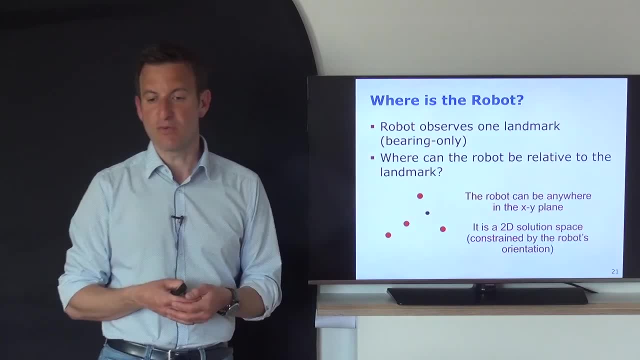 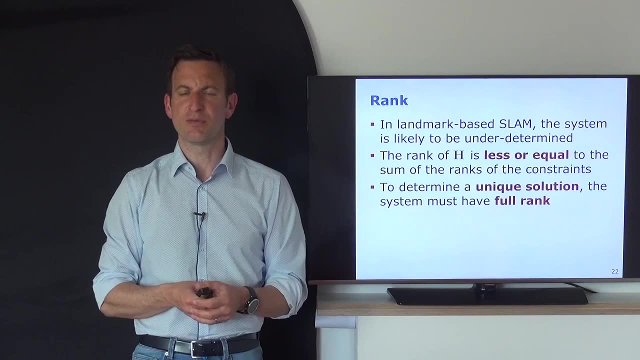 in order to fix the robot pose. This is kind of the minimum that we actually need, So I hope this example- although this was basically fixed- a landmark and estimating where the robot poses- has told you something: that we need further information than one single observation. 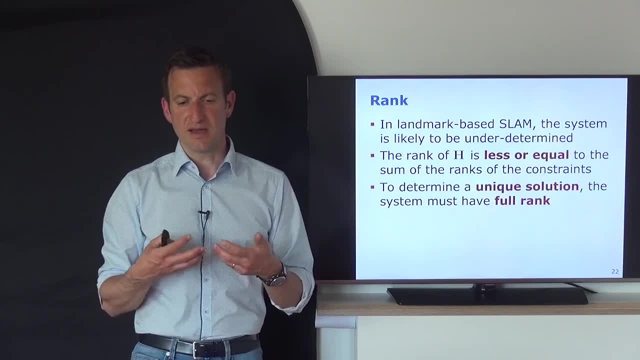 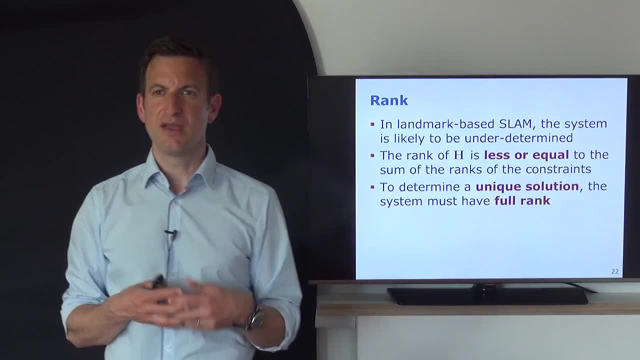 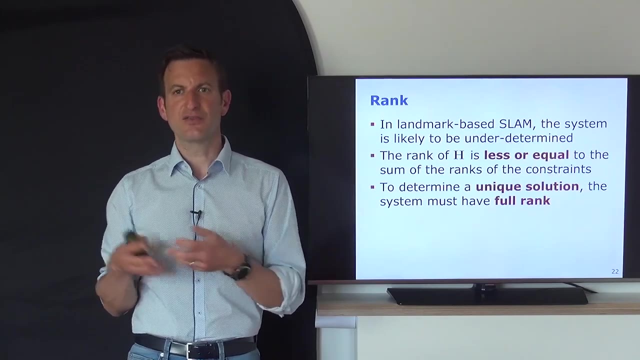 in order to be able to deal with the optimization problem in the context of graph-based SLAM with landmarks, And the rank of the observation here plays an important role. So the rank of H of any matrix is always less or equal than the sum of the ranks of the individual constraints. 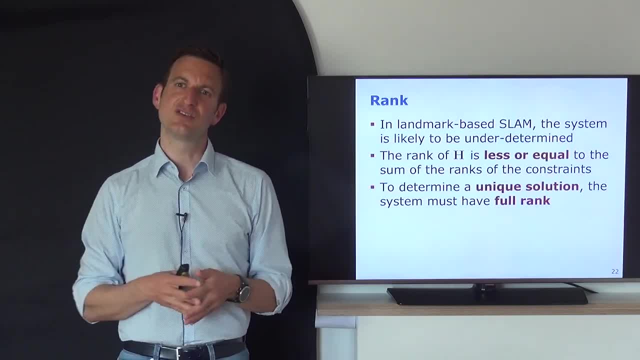 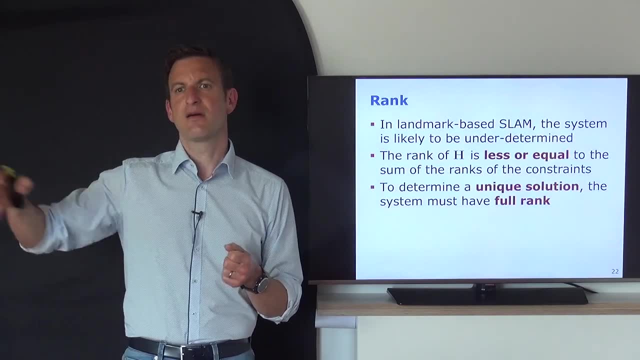 If you remember, H was built up by summing up the ranks of the individual constraints. So you will basically the rank of H will be smaller or equal than the rank of the individual observations. So that means typically we need to have a large number of observations. 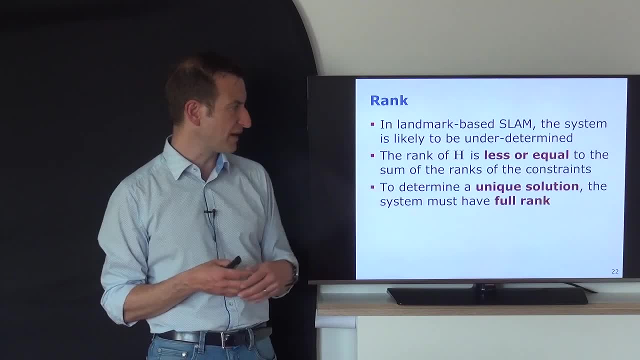 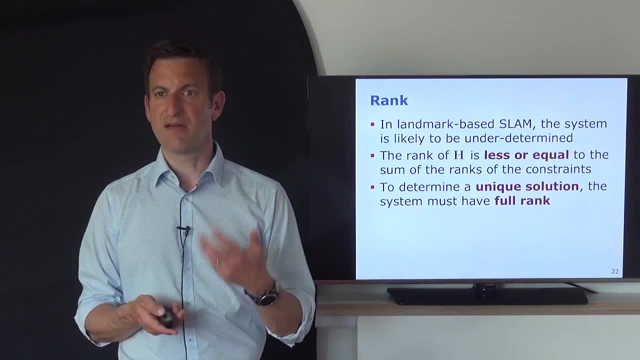 to actually make sure that H is full rank. Why are we interested in full rank? Because only then we actually obtain a unique solution, right? So we want to have a full rank, Otherwise we may not be able to fix all the parameters. 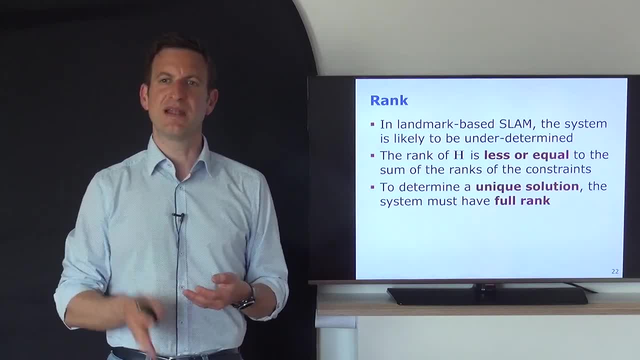 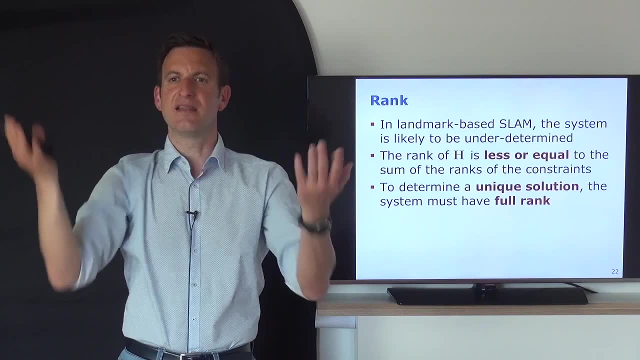 You can see this, for example, within bearing-only observation. If you've seen one landmark only once from one location, you only know where this landmark lies on the line, And any position on this line is a valid solution to your problem. So this is not unique. 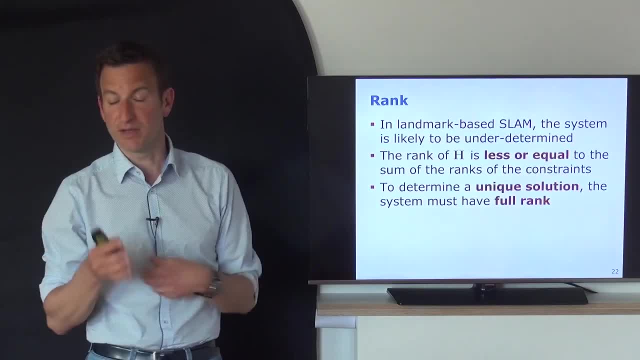 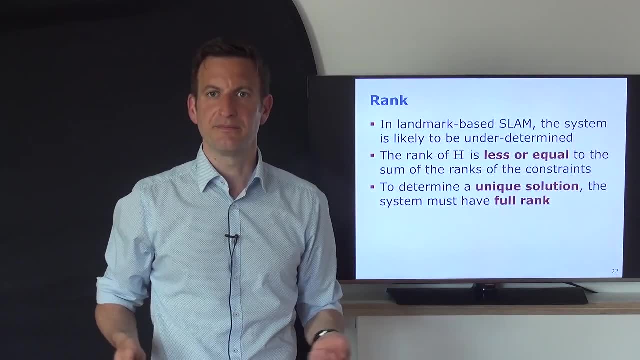 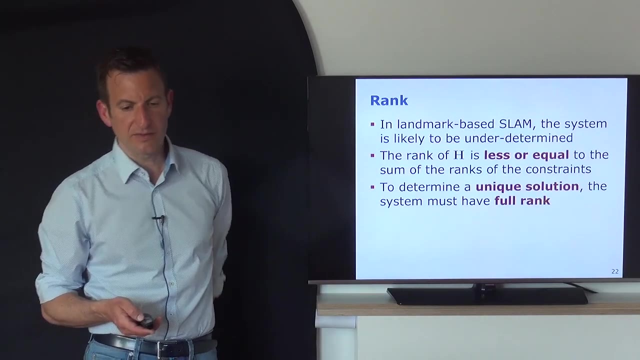 So you can't determine this landmark location fully, only constrain it to a line, And this leads to the problem that we have of having these constraints. that doesn't allow us to fully fix the the system that we have, in order to have a fully determined solution. 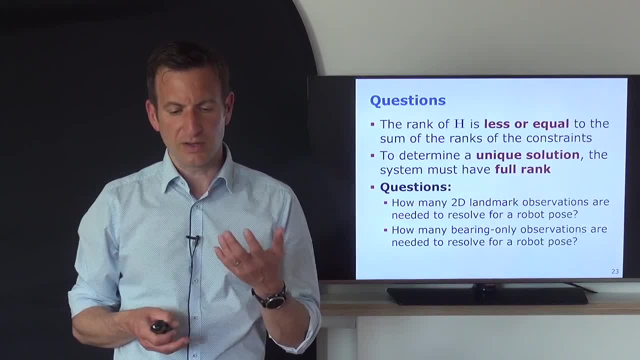 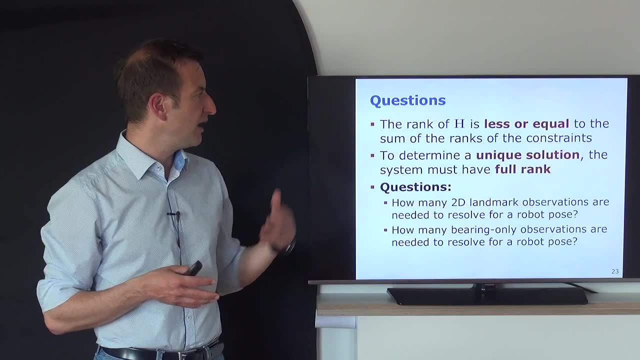 So a few questions. What So if the rank of H is smaller or equal than the sum of the ranks of the individual constraints and we need to have a unique solution in We need to have full rank in order to complete a unique solution. 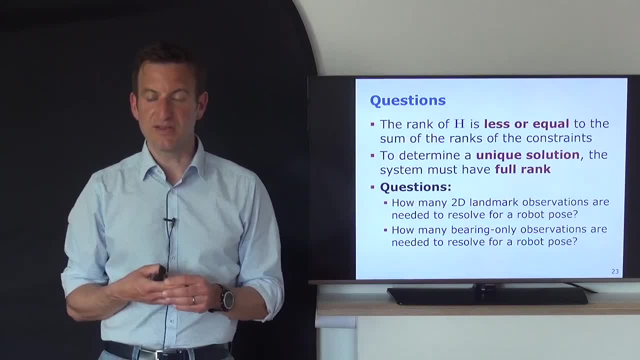 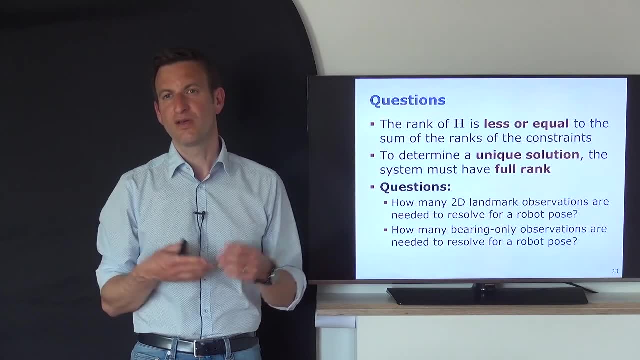 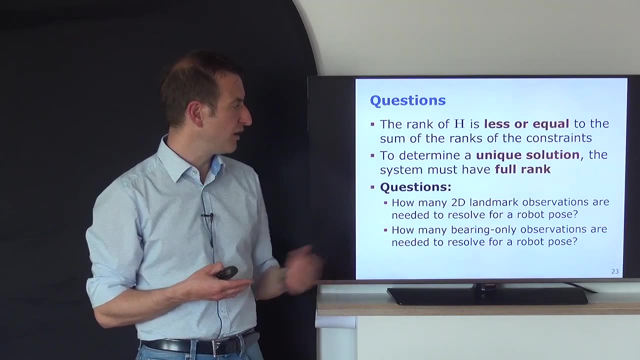 So how many 2D landmark observations do we need to resolve the robot's pose? And again, in order to fix a robot's pose, that what we had before- we need two observations, minimum of two landmarks. And if we are in the bearing-only case, 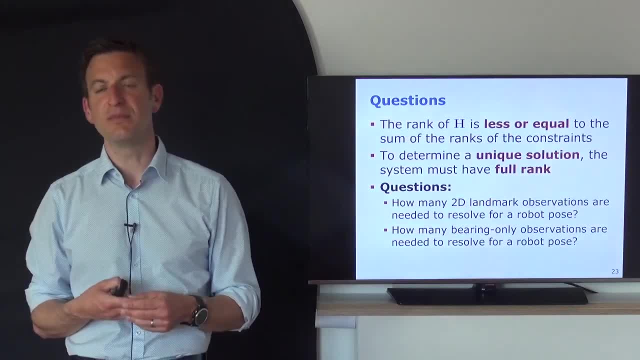 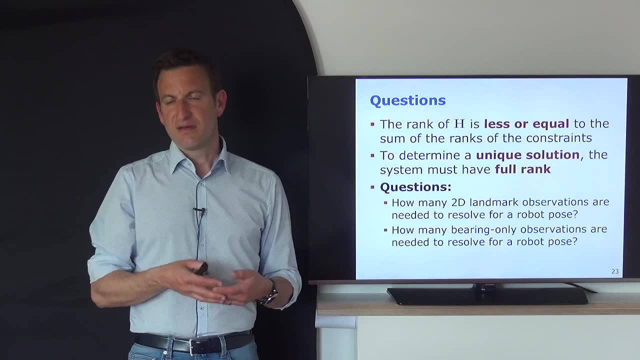 we need to have three as a minimum, Of course, assuming we're living in a 2D plane. If we are in the 3D space, then we need to adapt that, because we have six degrees of freedom to fix, But then depending on observations. 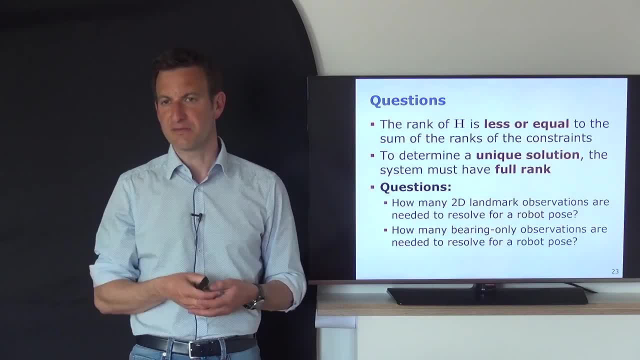 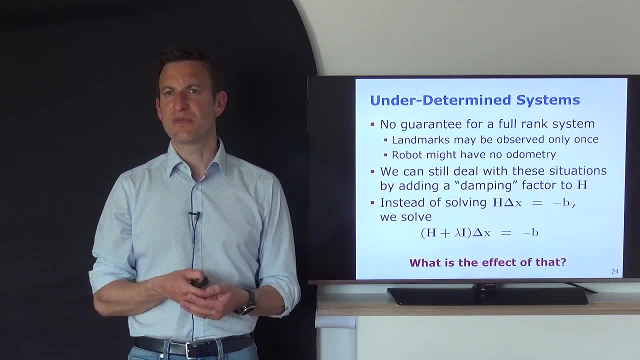 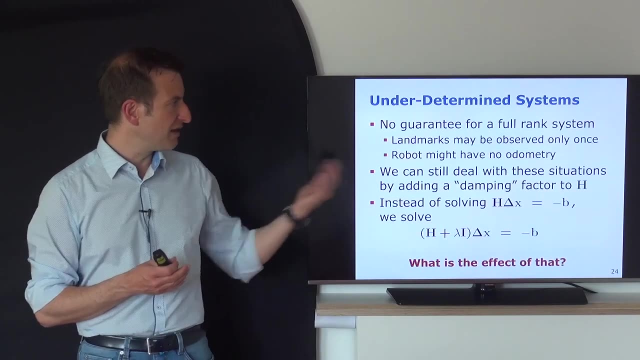 we may have two orientation angles, for example for the bearing-only case that we are fixing. Whatever we do in practice we often end up with an underdetermined, So there's no guarantee for full rank system, especially in this landmark-based situation that we have here. 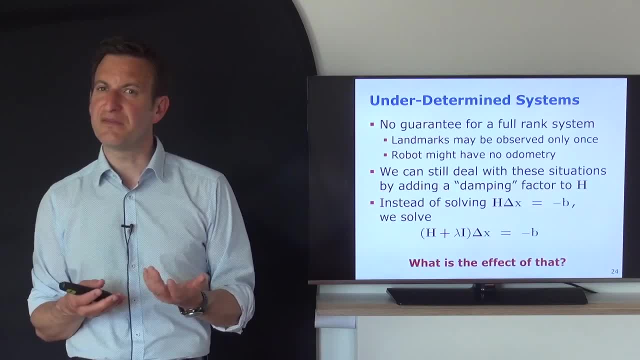 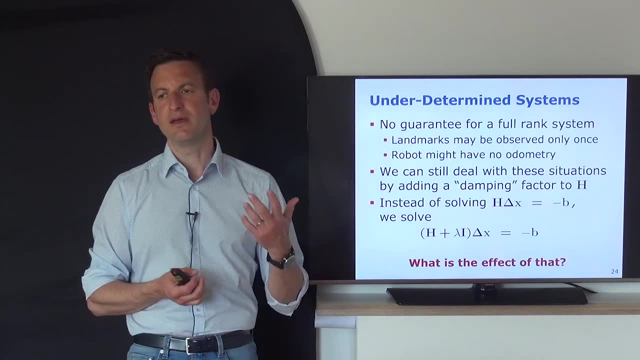 So landmarks may be observed, for example, only once. You might even have effects that the robot might have no odometry between two observations. If you have that case, you will suffer from this problem also in the postgraph. But if you always have odometry, 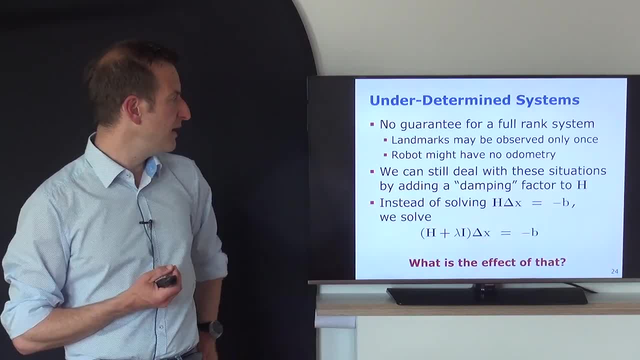 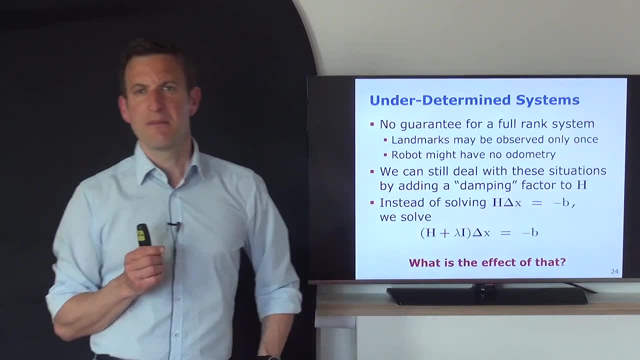 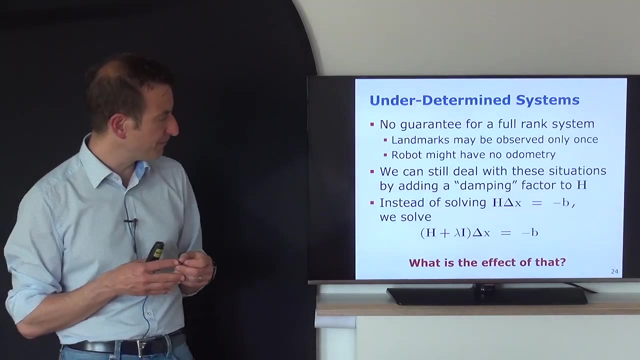 then that should be okay In the postgraph point of view. But there's still something that you can do in order to deal with such systems, And this is by adding an additional damping factor to H that is multiplied with identity matrix. So if you think about your original system, was H times delta, X equals minus B. 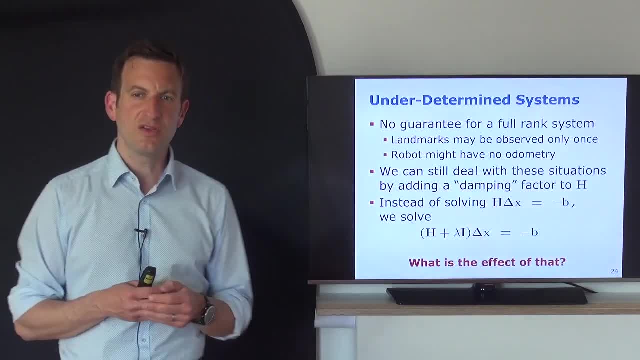 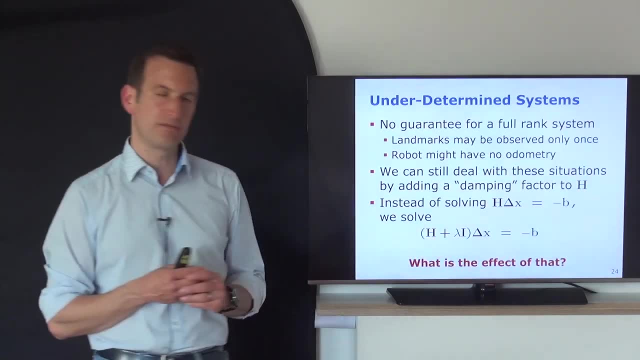 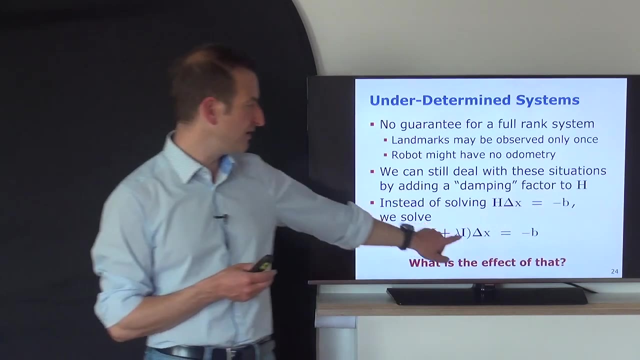 That was a linear system that you wanted to solve. What you can do now is you can add an identity matrix to this matrix H Plus a small scaling factor. So in this setup you're very likely to have a full rank matrix because the identity matrix has full rank. 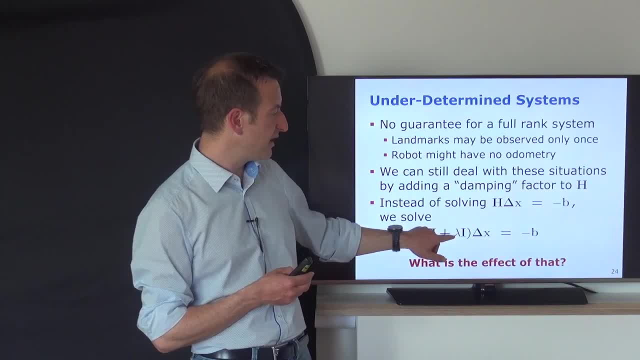 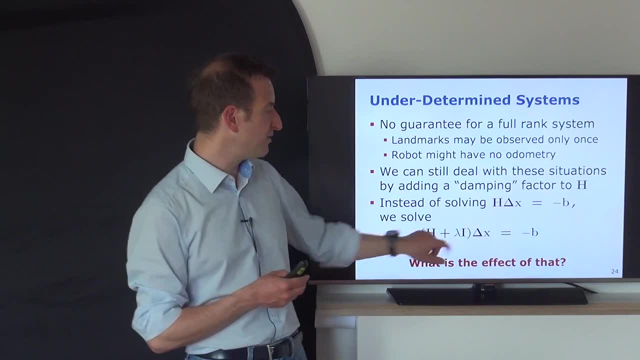 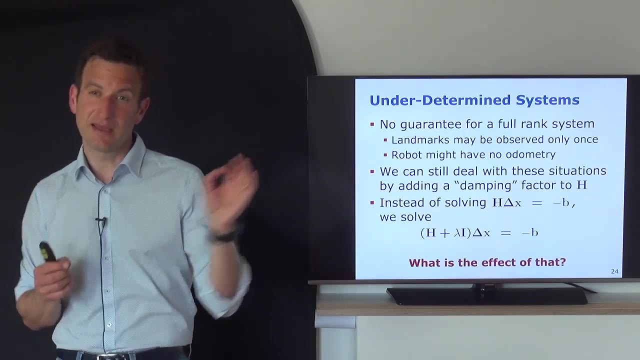 And so by adding, let's say, a small scalar times this identity matrix, this is likely to have full rank And if you make lambda small, you still have a full rank matrix and may not change the system too much. Although, again, if 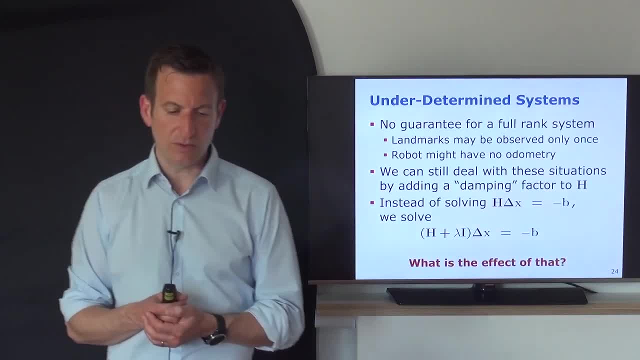 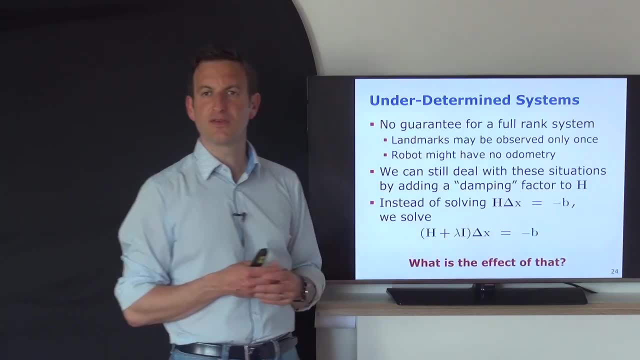 The lambda here gets very small. It doesn't mean that you have a well-conditioned system, but at least it has full rank, And then you can actually solve this system. And you may vary this parameter depending on the quality of your solution. 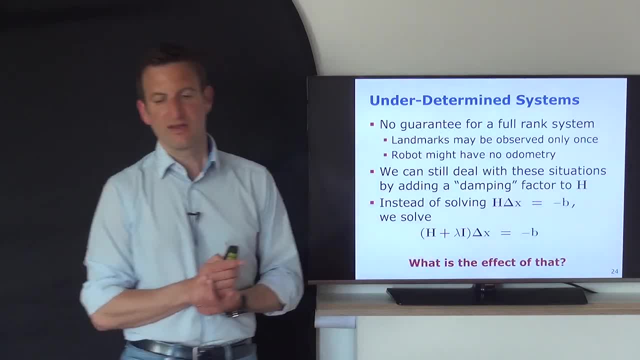 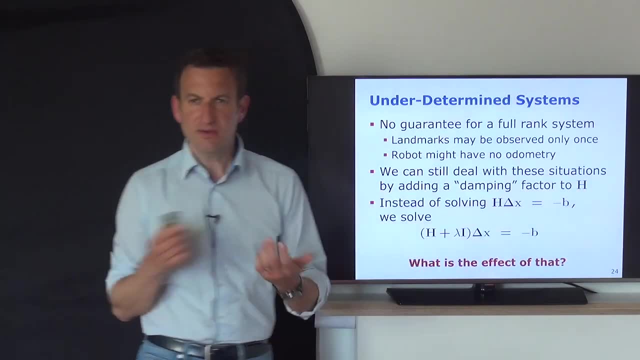 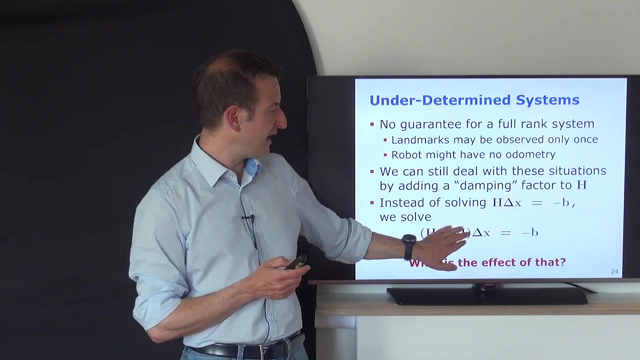 So the question is: what is the effect of doing this? Well, the interesting thing is that what you do here is basically a combination of two approaches, So H, delta, X minus B is what we are used for, And that is the result of a simple 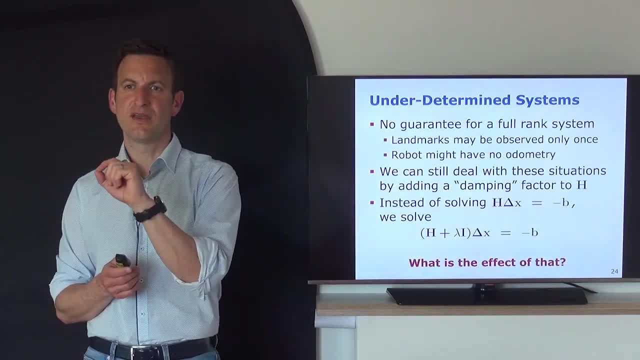 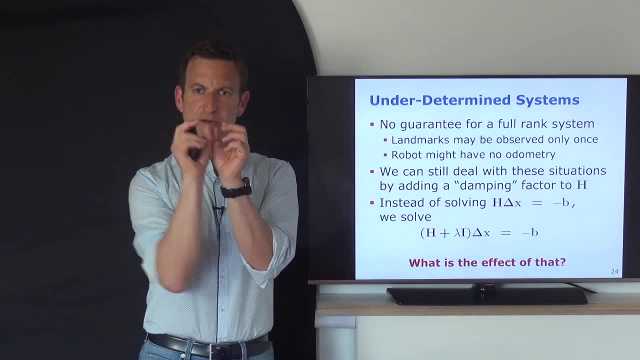 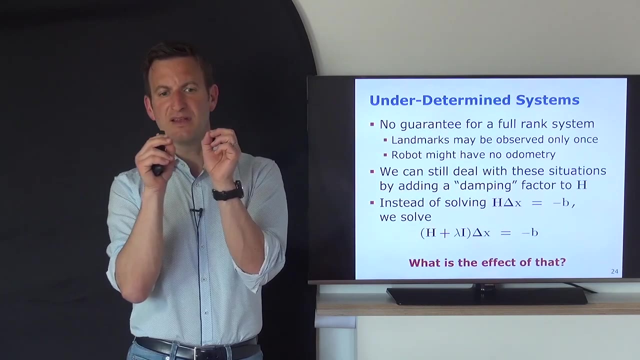 solution from Gauss-Newton. But if you think about delta, X equals minus B and you expand minus B, knowing that minus B is minus Jacobian, transpose information matrix the error and minus the error is the residual. What this basically does is you multiply the residual with the information matrix. 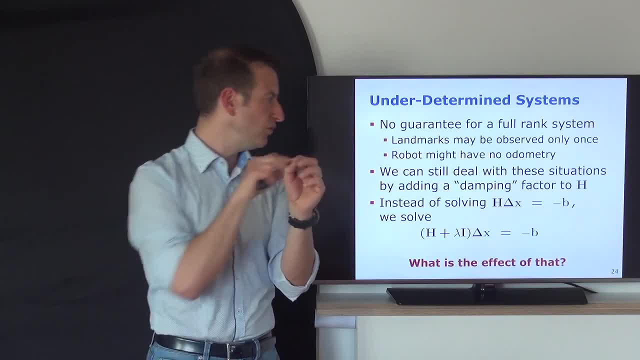 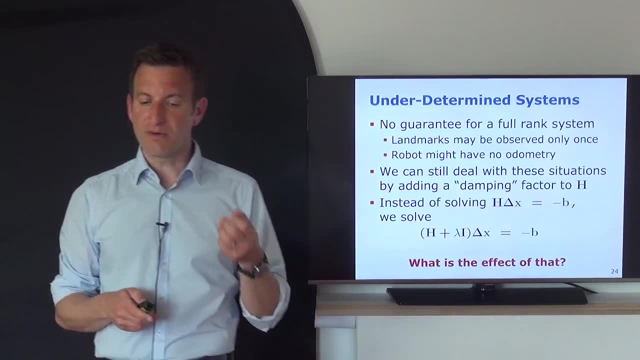 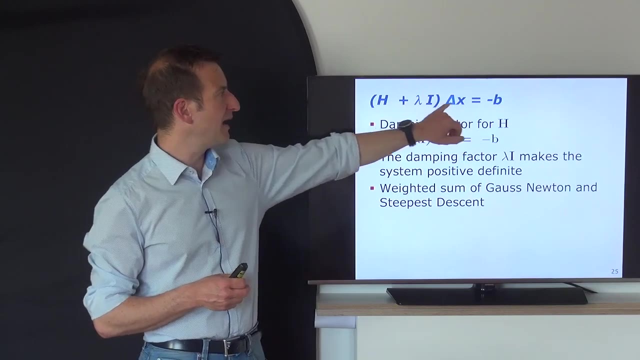 That means you scale it based on the importance, the residual vector, into the space of up, into the space of updates of your parameter in your parameter space. so it's a form of steepest descent that you're actually performing. so you can see that solving h plus lambda i, delta x equals minus b, is a combination of gauss-newton and a steepest. 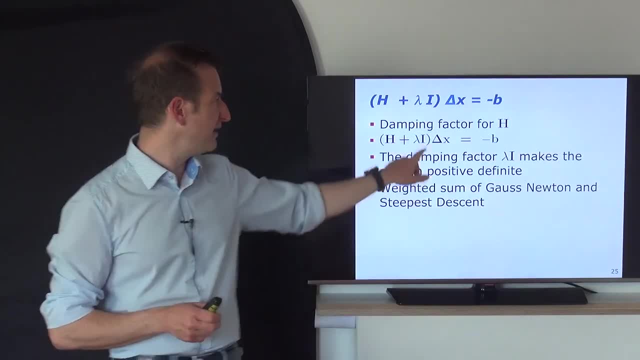 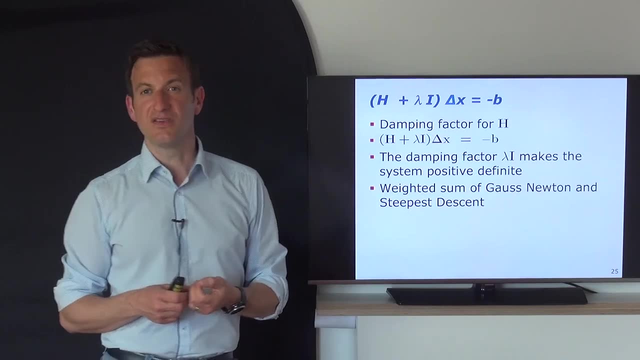 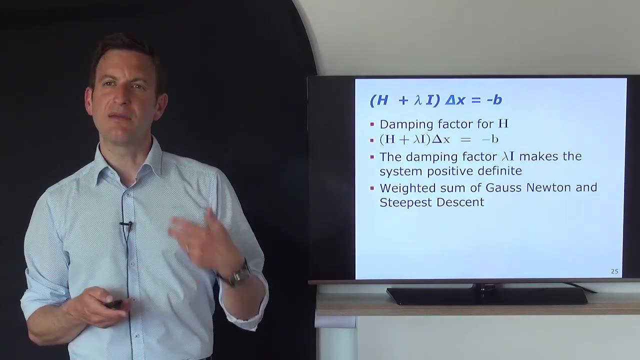 descent approach. so you're basically combining both. depending on the the scale parameter here you're saying how strong the steepest descent part of that actually is, and with this this is what is called the living back marquardt approach- you are actually able to deal with such systems. 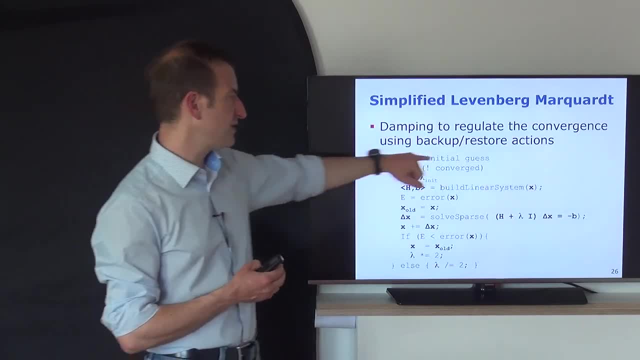 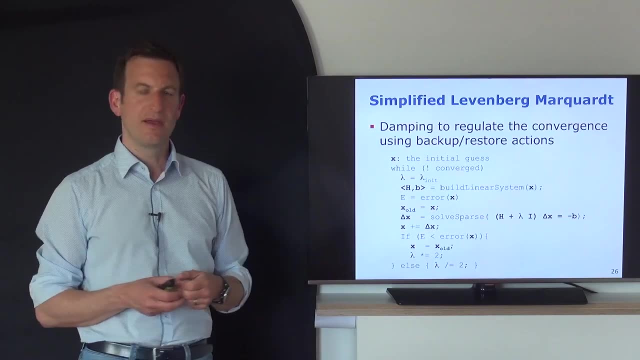 which are underdetermined. so how does it work in practice? so you have an initial guess of your solution x and then, while you're not converged, you have an initial damping factor you start with and then you build your linear system: compute h and b, compute your error vector, you start. 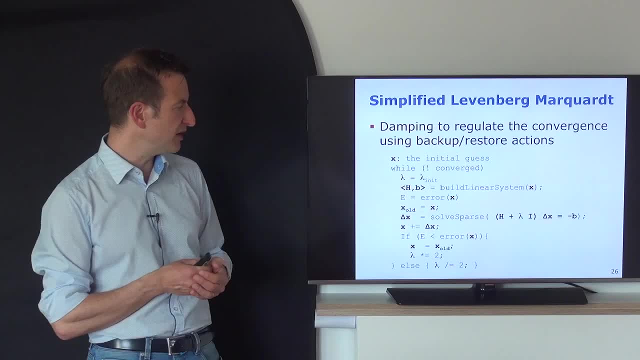 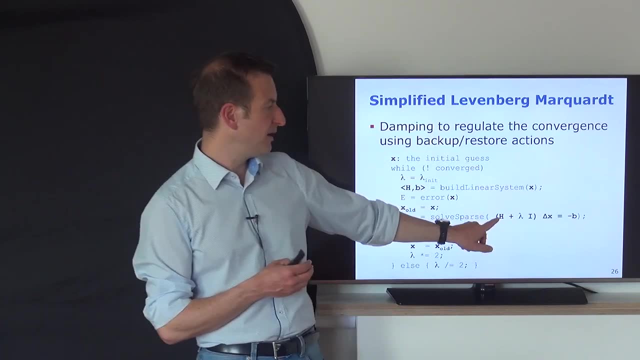 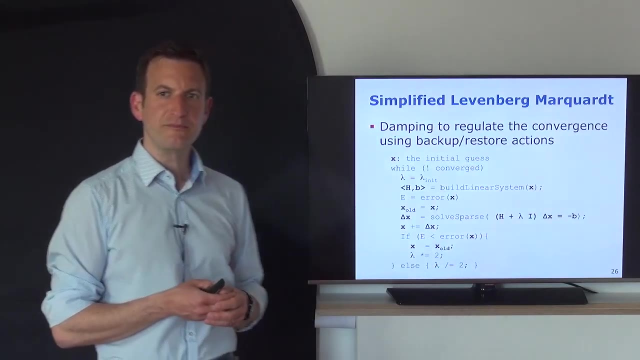 with your error vector and then you store your error vector to monitor if your error increases or decreases and how you change your, your damping parameter. and then you solve the sparse system. h plus lambda i, delta x equals minus b. for some sparse solver that you're using, 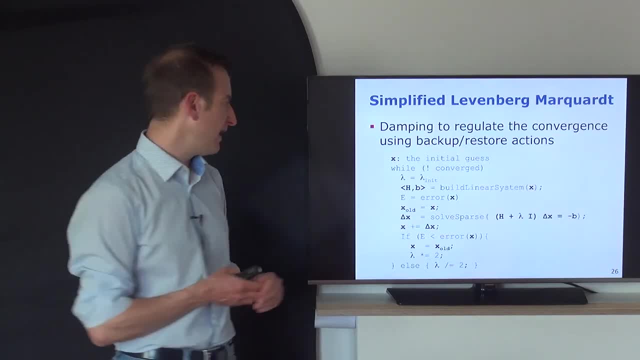 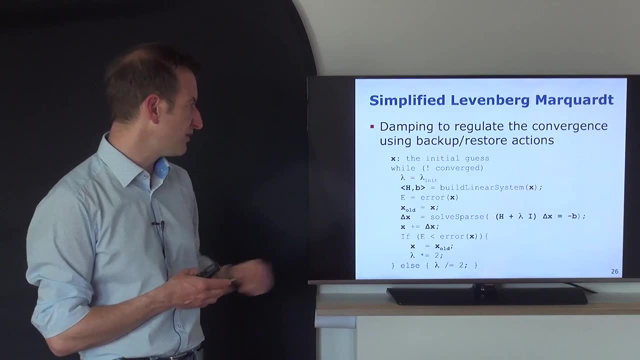 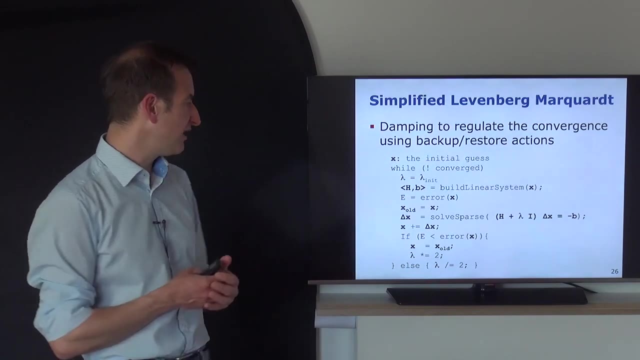 and then you get your delta x, you add your delta x to the solution and then you check: is e smaller than the error of this new solution is the error that we had before. if the if this is the case, then i say, okay, i'm, i still have. 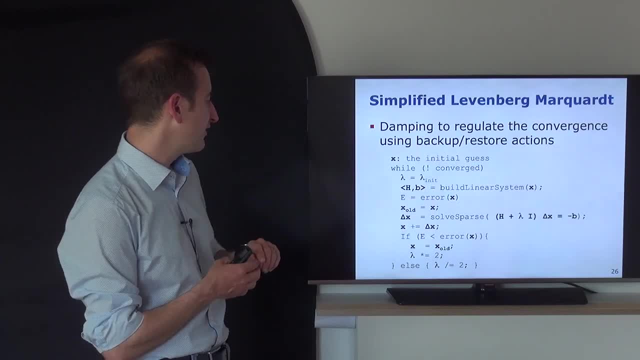 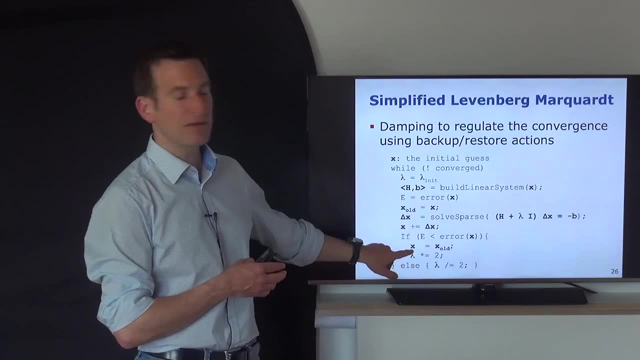 improved my solution, so my no, sorry. in this case, um i, the error is increased because this was the previous error and this is a new error, so the new error is larger. if this is the case, i'm recovering my old post and i'm actually increasing my damping factor. make the damping factor twice as large. 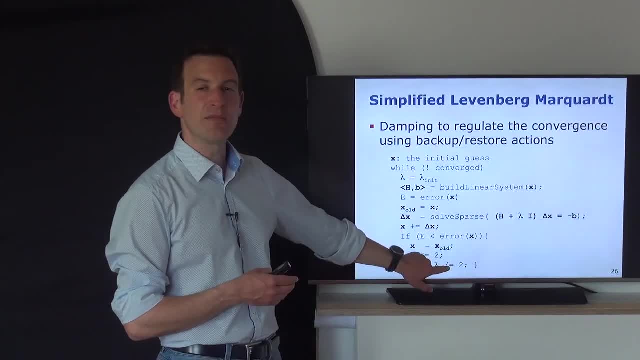 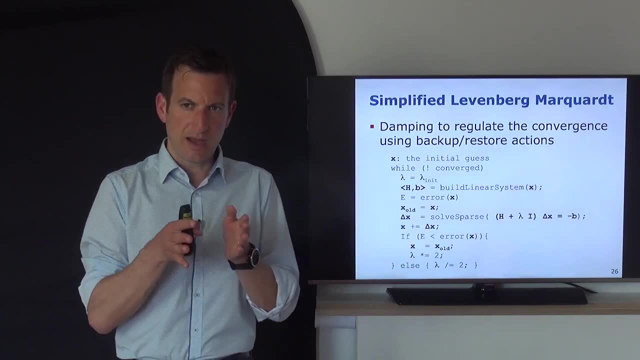 and if there's not the case, if i decreased my error, then i'm actually reducing my damping factor and then i restart this process. it so what happens is when i can improve my solution, i'm actually reducing the damping factor. whenever i increase my error, then i'm recovering the old pulse and increasing my damping. 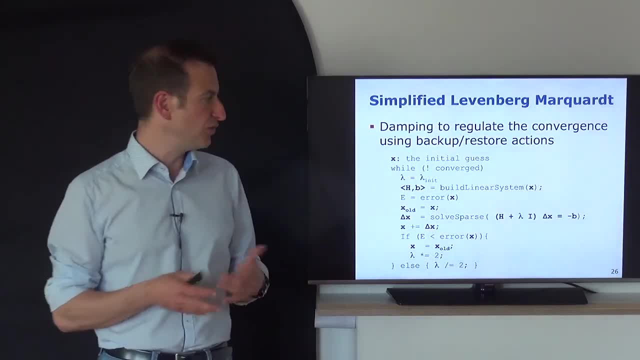 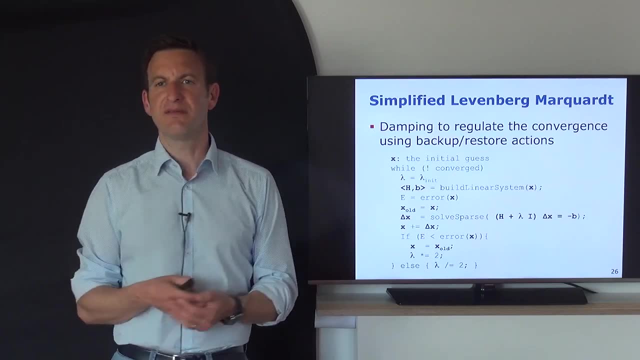 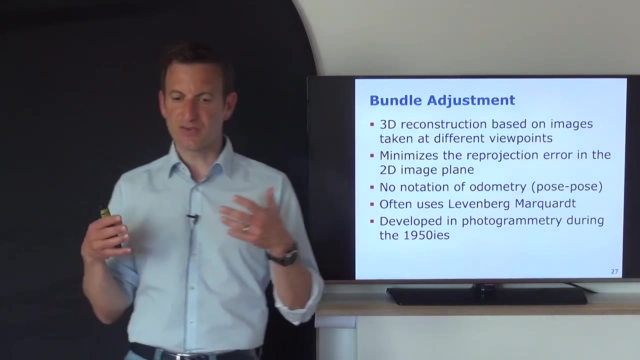 factor. so, in order to come as close as possible to a solution that approximates h, delta x equals minus b, and this is also an approach that you typically find when using a bundle adjustment solution. so bundle adjustment is basically um slam based on images. so reconstruction based on images, where you just have a collection of images and feature point. 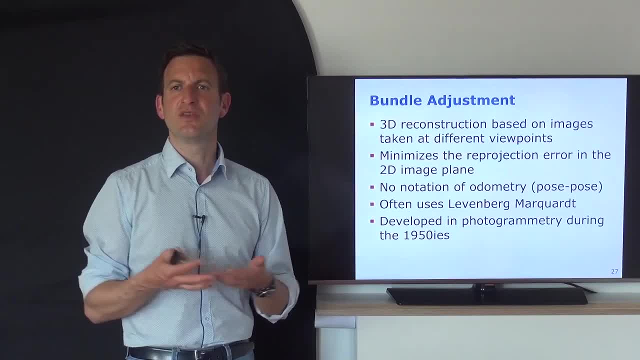 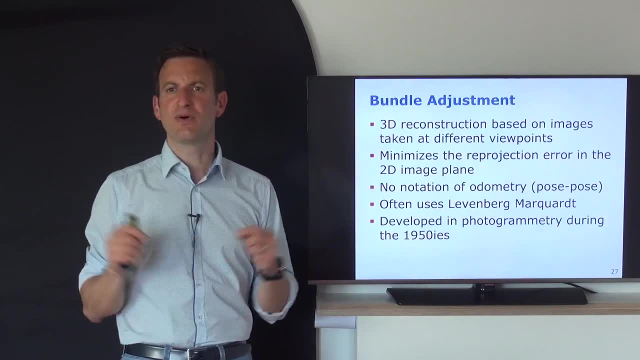 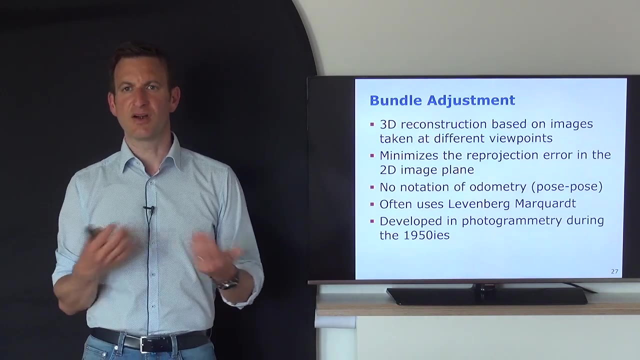 that you observe from the environment. so bundle adjustment, for example, assumes, doesn't assume that you have odometry information. you just have an unread set of images where you extract feature points. you assume to have correspondences between those feature points and then you want to estimate the camera locations and the feature points in the environment in 3d. and what this approach? 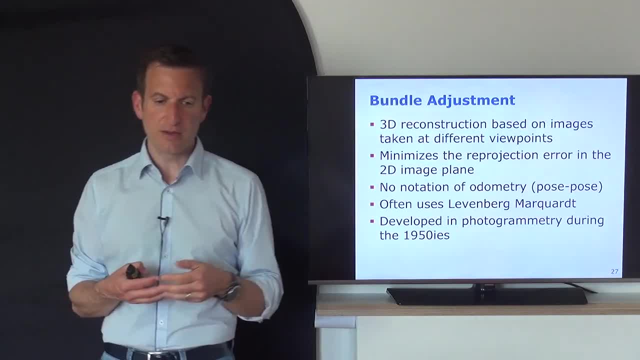 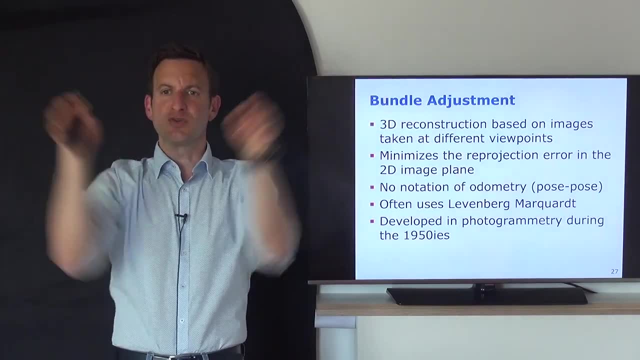 typically does. it minimizes the reprojection error of the feature points into the 2d image plane. that means you estimate where your cameras are, you estimate where your 3d points are, you project the 3d points into the 2d image plane and then look to the discrepancy between where. 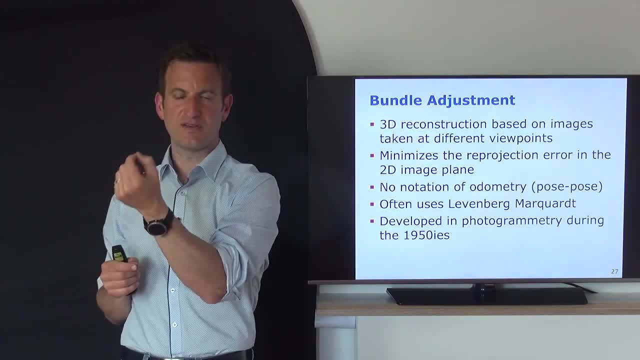 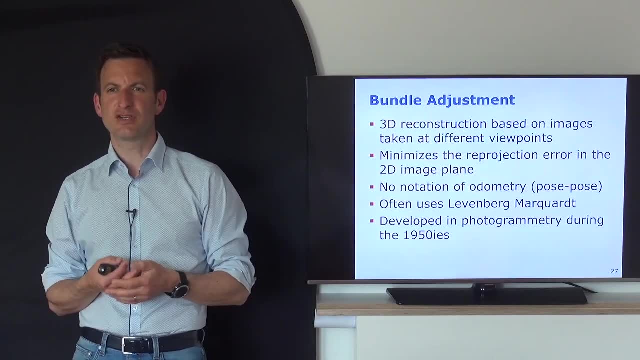 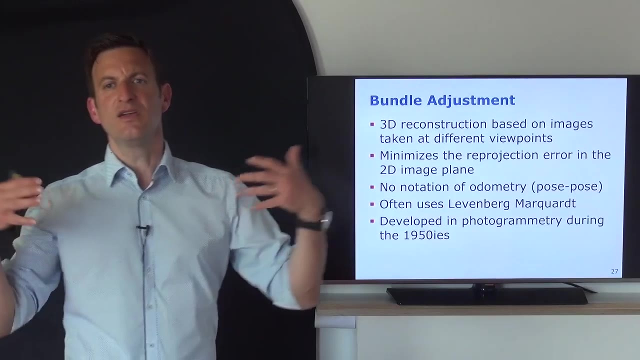 the feature is measured or the point is measured and where the feature should be. given your given this reprojection, and especially if you have no notation of odometry, you more frequently suffer from these underdetermined systems and need to address this in an appropriate way. you need to 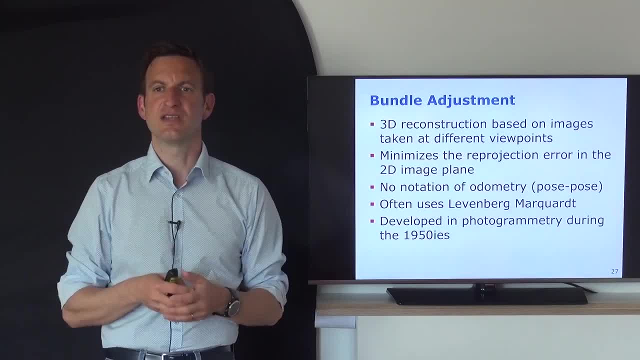 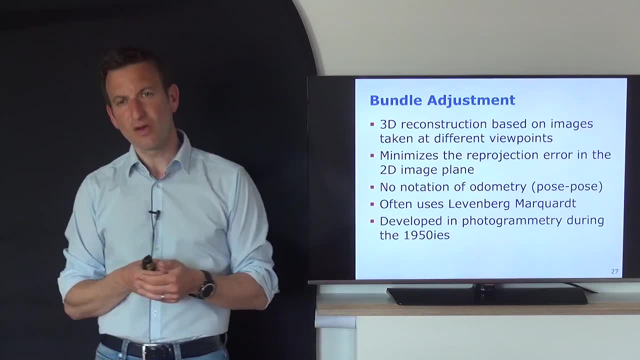 have enough observations of what's going on in the environment and what's going on in the environment, the same environment, in order to have actually connected graphs. otherwise your graph actually breaks up into several places, and solutions to this problem exist since quite a long time, so since, let's say, approximately the 1950s, and photogrammetry approaches have been developed. 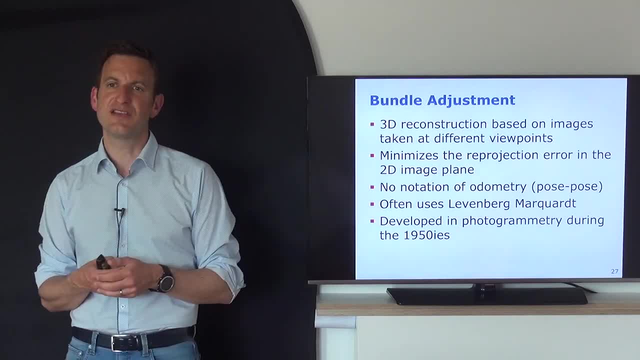 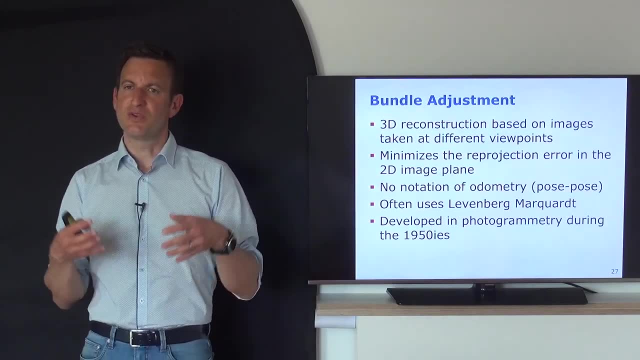 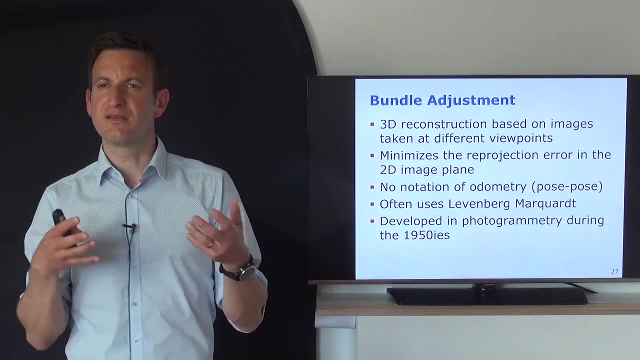 for that, and you can see this as a special case of the graph-based slam problem with landmarks in the graph-based slam. we typically incorporate more information to this- odometry information, some other additional information that you can include into this- but structurally they're actually very, very similar problems. so to sum that up, what we have discussed here is basically an extension.